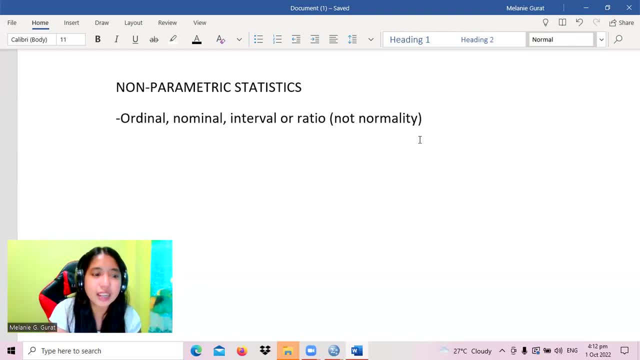 Therefore, we will be using parametric tests. Now, what if our data, If our data is not interval, so let's say, for instance, it's an ordinal data or it's a nominal data. So therefore, again, we cannot use parametric tests, but things that we have what we call as non-parametric statistics that will still allow us to answer our inferential questions. 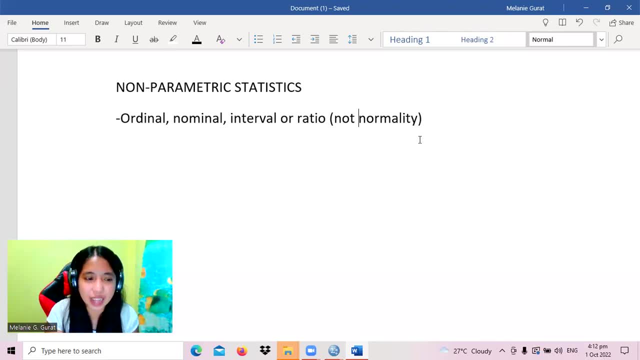 So, just like with the question in a parametric test, like questions on comparison questions, Questions on relationships, questions on prediction, this can also be solved using a non-parametric test. But because the claim is that parametric test is more powerful than non-parametric test, the first choice that we are trying to do or to use is the parametric test. 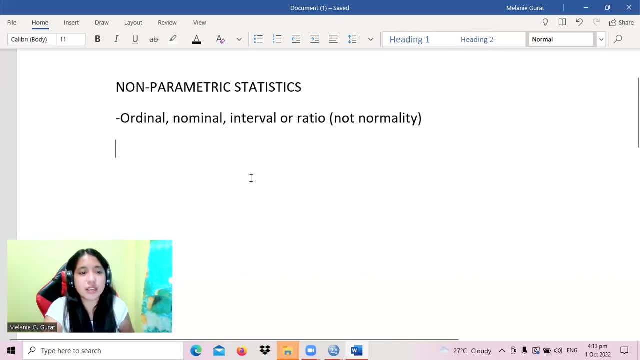 Now going back to non-parametric test. So, aside from saying that This can be used for ordinal data, nominal data, interval or ratio, there is also, of course, some- what we call this- characteristics that we need to consider. 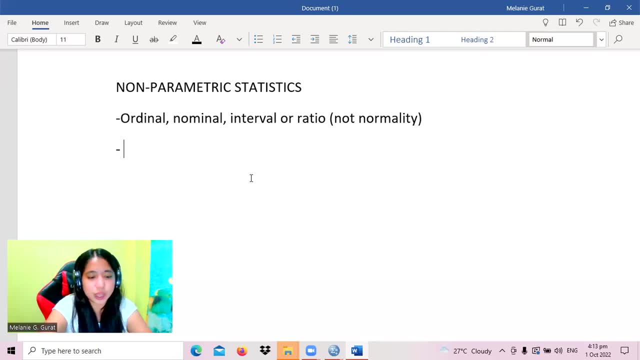 Just like if we are using this, it means that we can use the median as our location parameter. So remember that when we We also use our parametric test, we are using mean and standard deviation, But for non-parametric, the appropriate is also median. 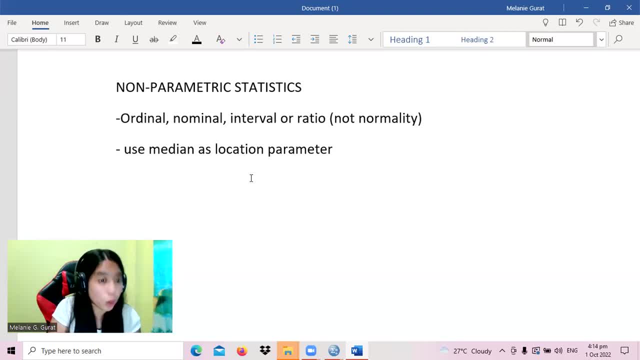 Because, if you can still recall the appropriate- also measures of central tendency, given the data, If our data is ordinal or if our data is at this interval but it is not normally distributed, the best or appropriate measure is the median. So it is just, of course, right to mention that when we use this, we are using a median as the location parameter. 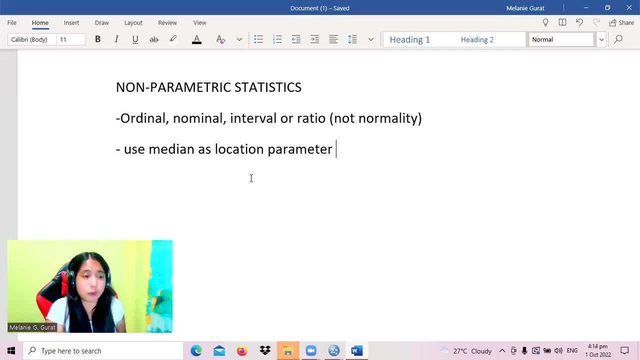 So it is. it can be used whenever we have also skewed data or not normally distributed data, which means when we have two groups that will be compared. It is okay if the one group is is twice or thrice larger than the other group. 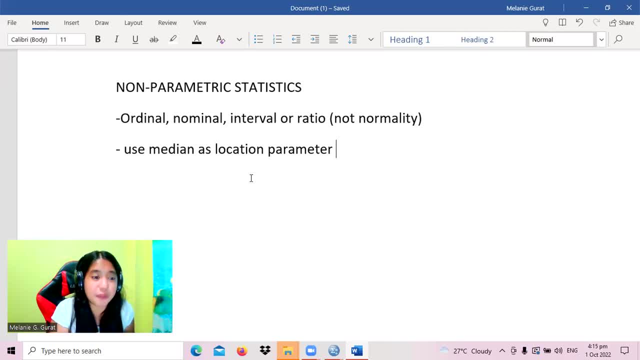 So it's not really a concern or an issue for a non-parametric test, even if it is not equal or it's not approximately equivalent. So we also, of course, mentioned that this is a weaker statistical power than a parametric statistic. 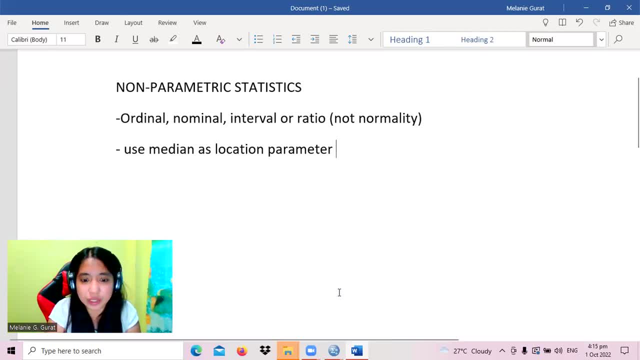 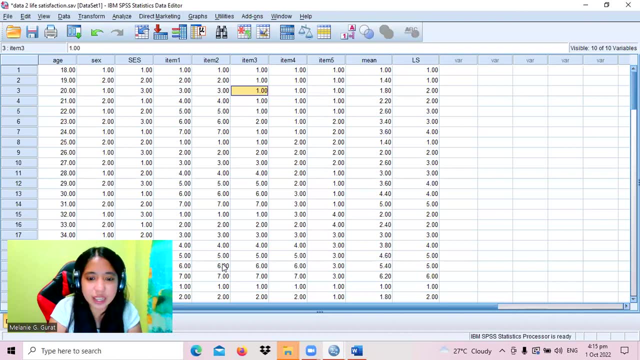 Now I have here a data on level of life satisfaction. So this is the data. So, if you can still recall, this data is obtained in the questionnaire on life satisfaction, asking the respondents for the profile variables like age, sex, socioeconomic status and, at the same time, 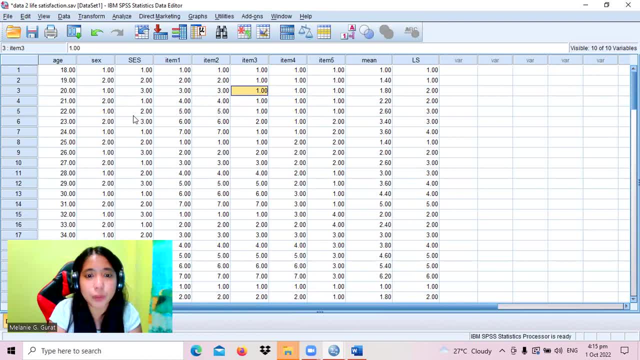 I'm also asking them to rate The items from. originally it's one to seven. So still, this is still one to seven, But instead of using the sum, which is the? what do you call this? It's the main. it's used, of course, to guide us in how to interpret the data. 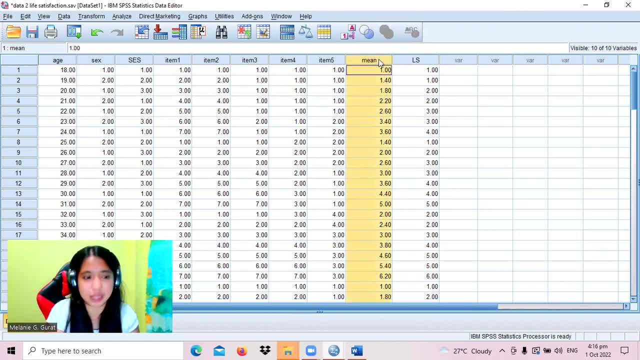 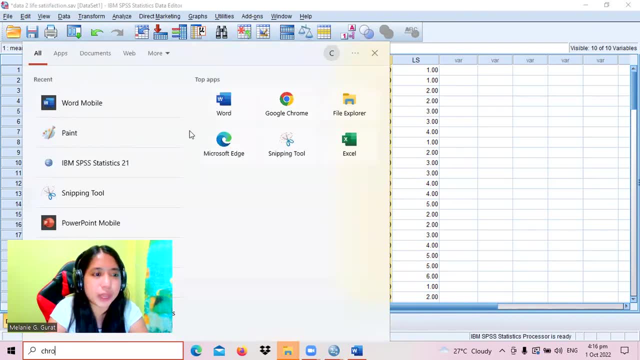 I replaced it with With the mean. I just replaced with the mean, So just to maybe have an idea about that. maybe we can go over with that questionnaire. So let us see. So if we can use that questionnaire. 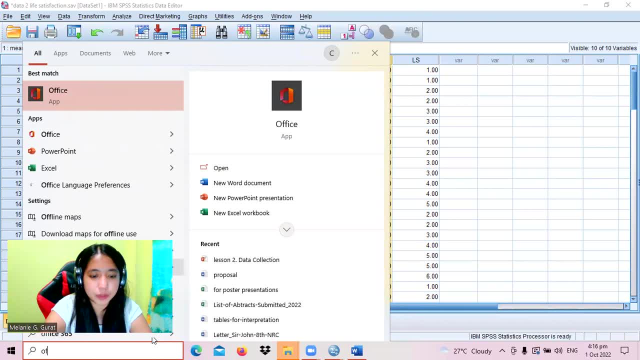 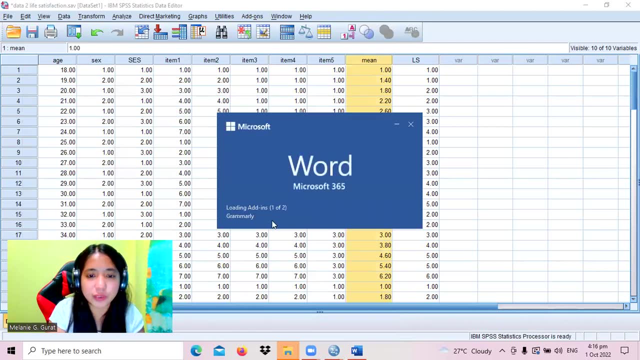 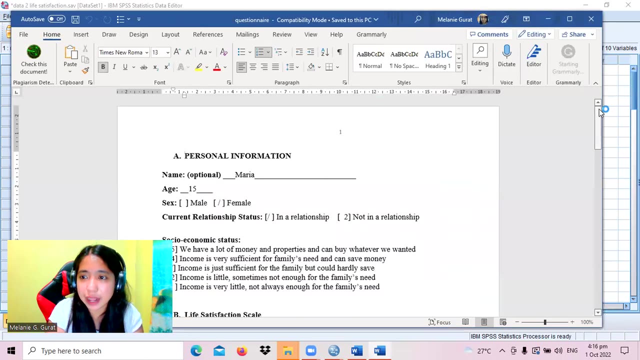 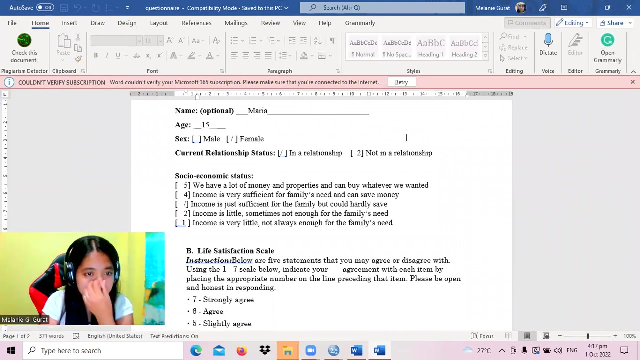 So let's go over our, Let's have a look of that. So this is the questionnaire that I am. So this is the questionnaire that I am mentioning. So we ask for age for sex, for current relationship status. 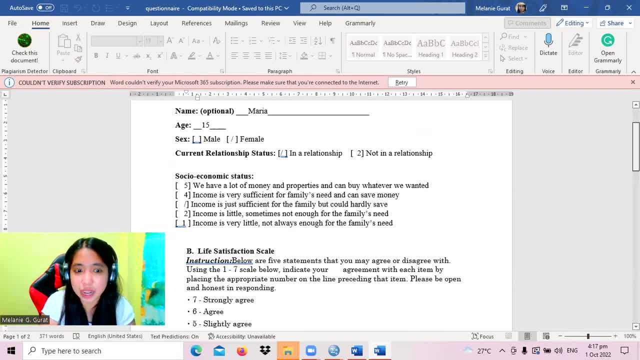 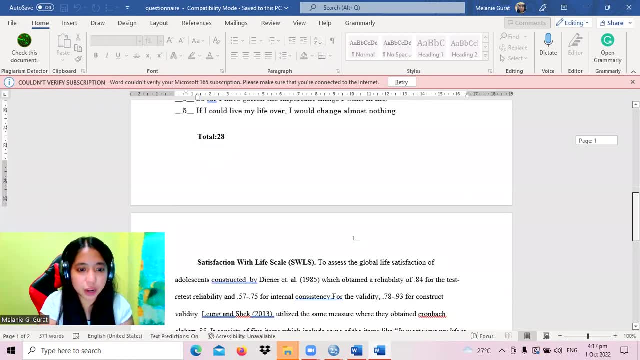 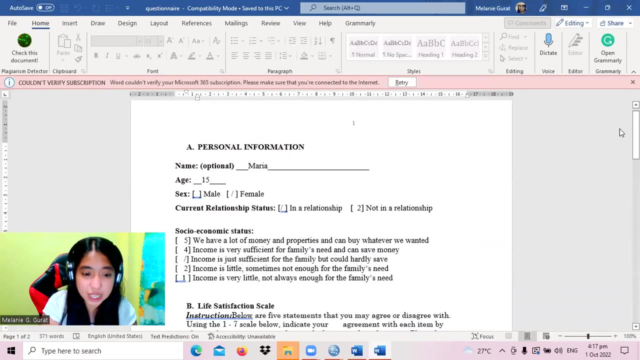 and socioeconomic status, And then for the life satisfaction. This is for the items. So we have five items And originally it is from diner, So but, as mentioned, instead of using the sum, I considered using that mean, Or we can also use it any way. 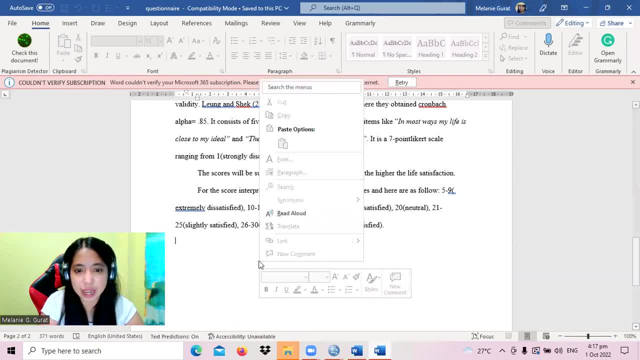 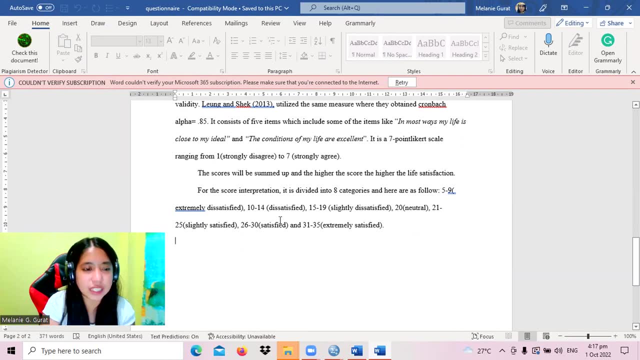 The guide is also being presented, like here, So let's see. So: if it's five to nine, it means it's extremely dissatisfied. If it's 10 to 14, it is dissatisfied. Let's go back here. 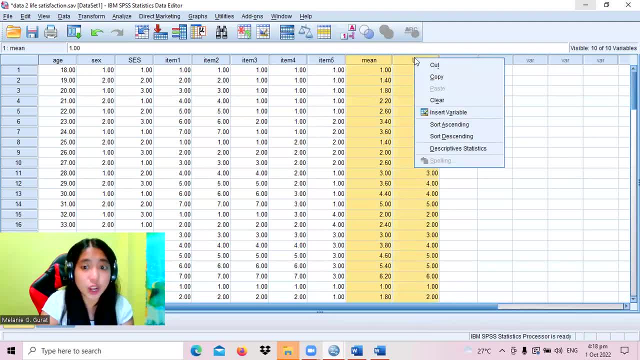 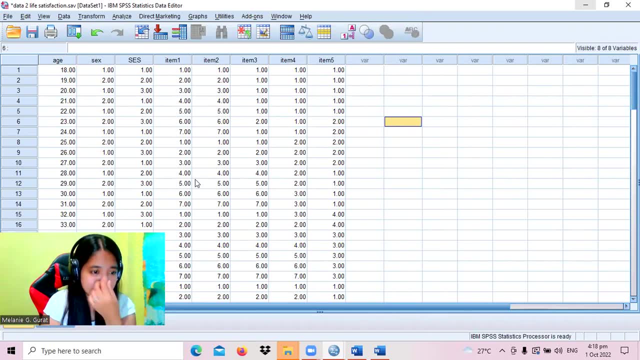 Let's just remove the mean and LSN. Consider the original questionnaire. So, given this data, our objective is to first answer Or to get the sum by, of course, computing for the sum of items one to item five. So the data here is age, sex and socioeconomic status. 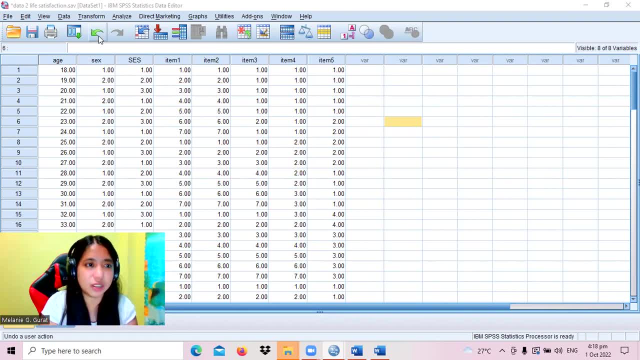 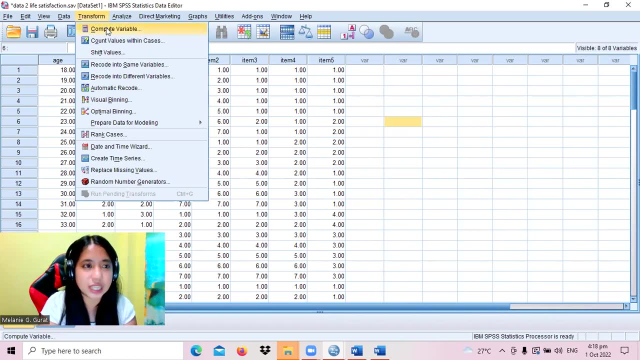 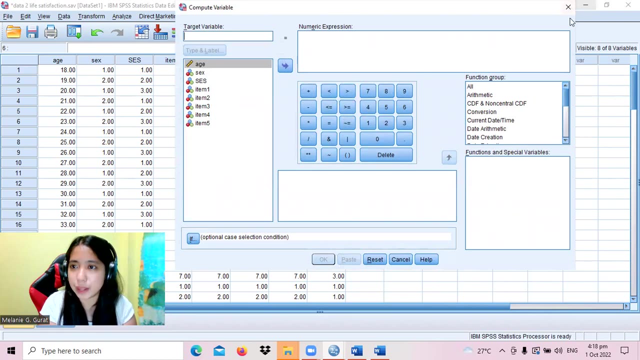 And the responses in item one to five. That is the just compute for the sum. So you can do this using Microsoft Excel or you can also do this here. So transform and compute the variables. Okay, and let's see. so, let us. 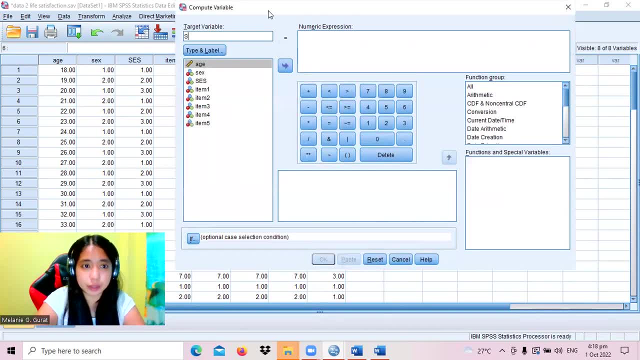 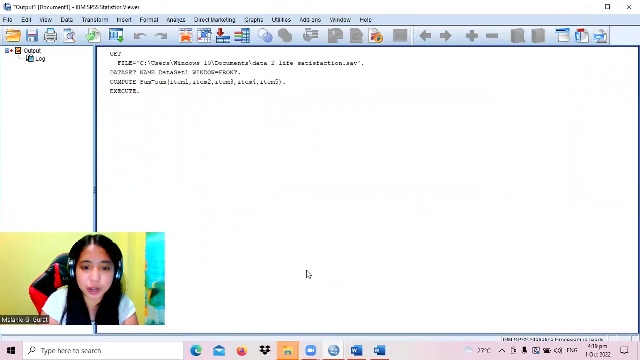 get the sum and then compute for the sum here. so sum open. parenthesis copy each item: item 1, item 2, item 3, item 4 and item 5, of course here. so this is the output viewer, so it is where we can see the output. 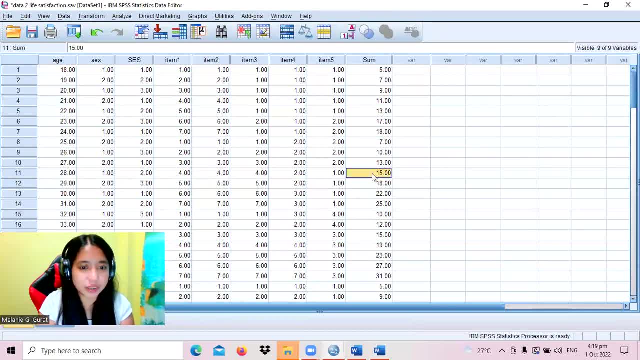 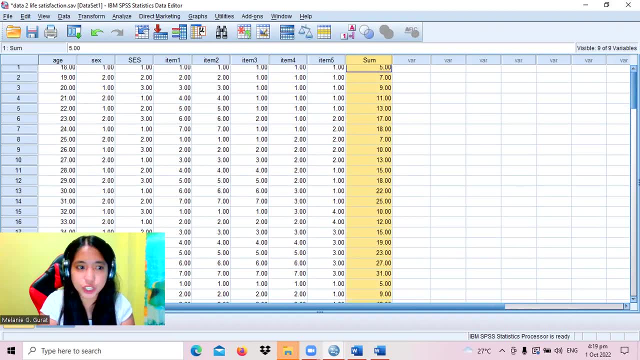 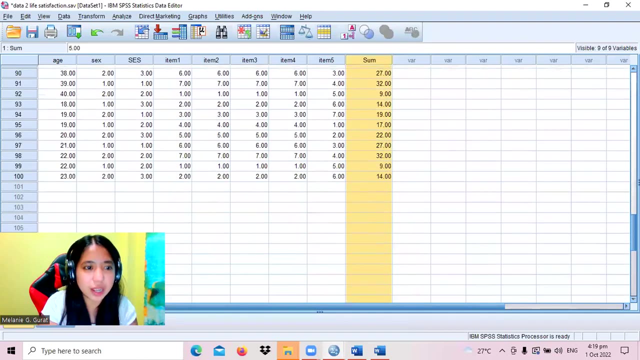 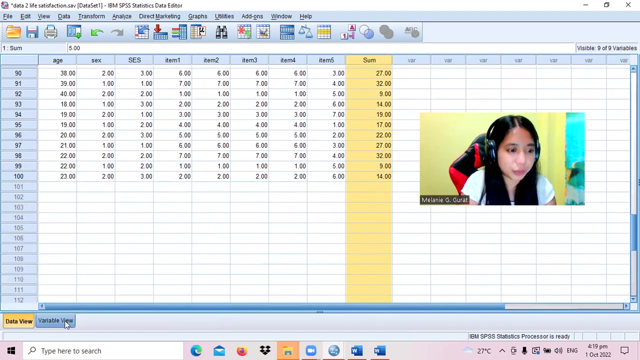 so let's go back. so of course, here after generating the sum. so we have an additional variable which is the sum. so just to check the number of respondents, so we have 100 respondents, but later if we will be checking also for, let's say, for the variable view, 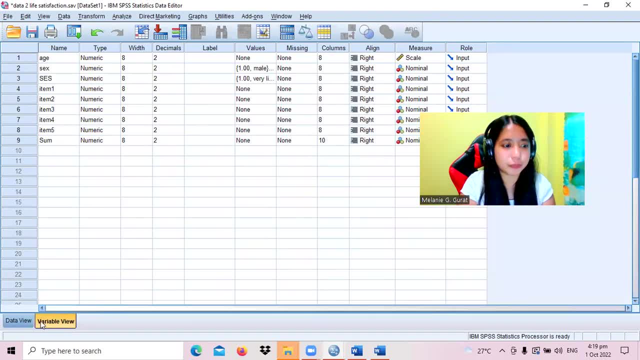 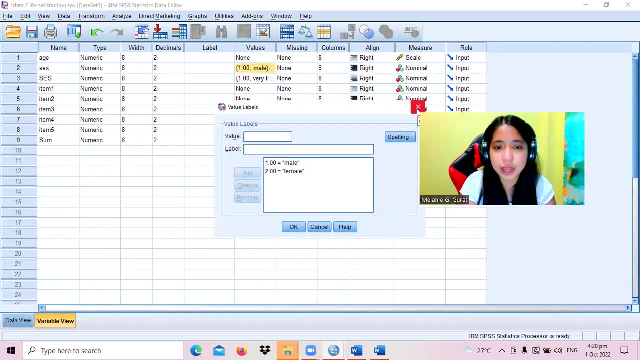 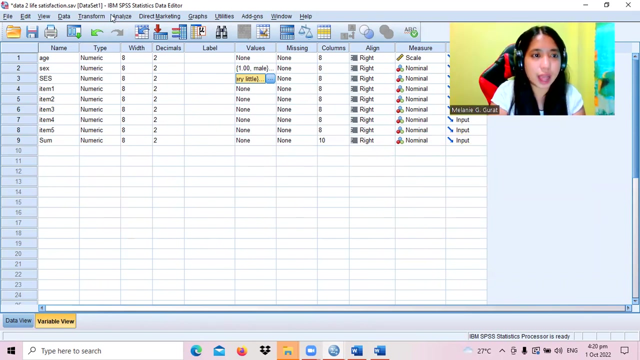 so we have, of course, the scale. the value 1 for male, 2 for female, and socioeconomic status is: 1- very little, 2- little and 3 is the suggestion. so let us generate the number of respondents to analyze group according to the profile: descriptive frequency. 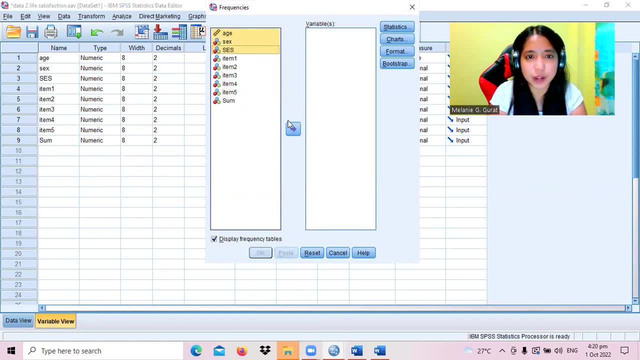 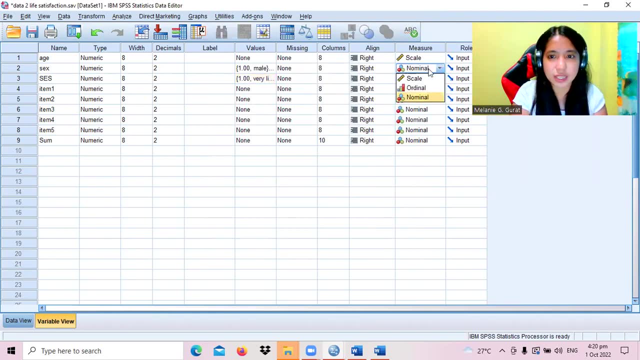 so let's just also get the profile. so let's go back here. let's just classify first the measure. so sex is a nominal data, socioeconomic status is an ordinal data and these are all ordinal ordinal data. so the individual items, though it's um, it is treated as its score. 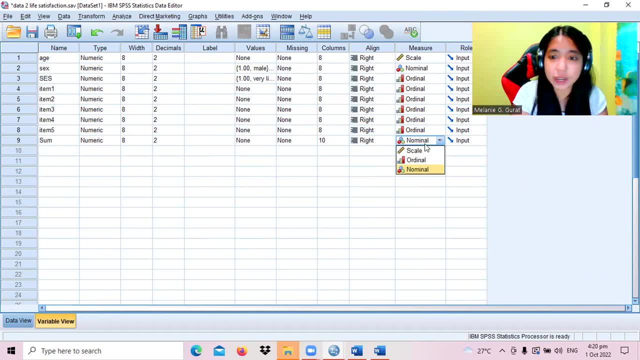 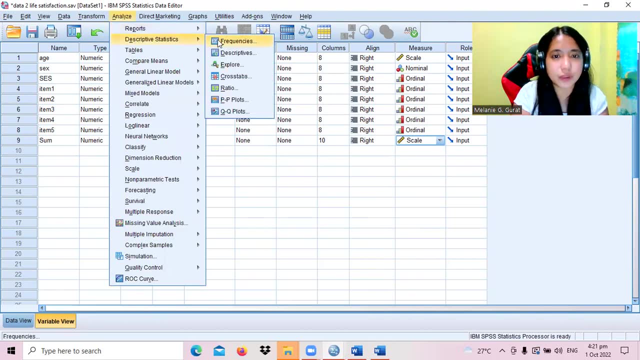 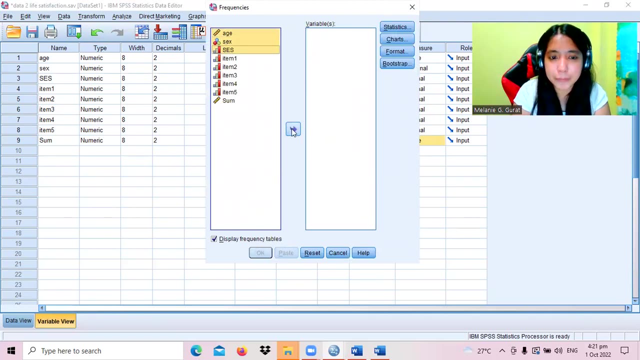 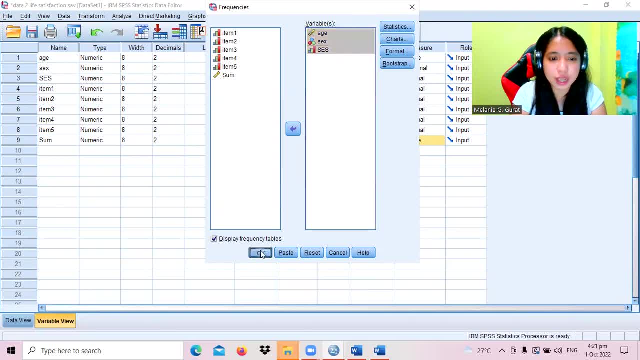 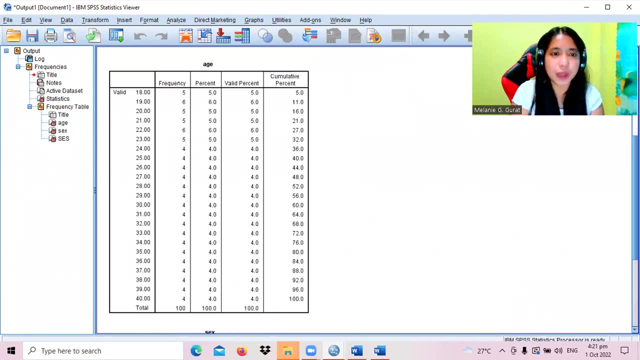 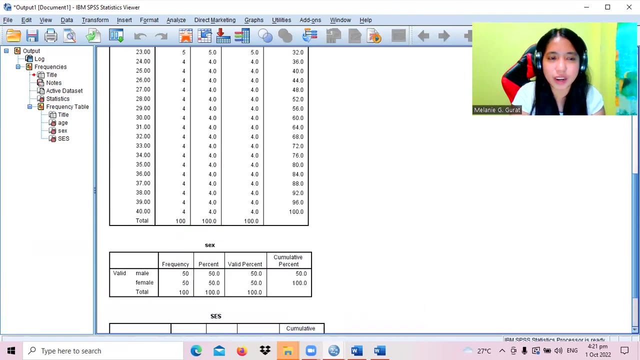 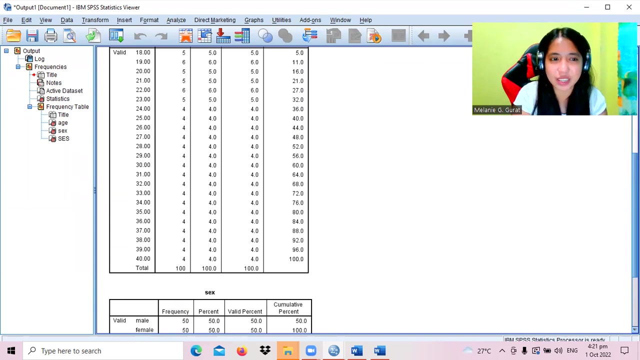 So we transferred our variables and click the page. So we have several variables here, which means later we have to do something first with our data and then we have to group it, Because of course we are not concerned of grouping our results for each of this page. 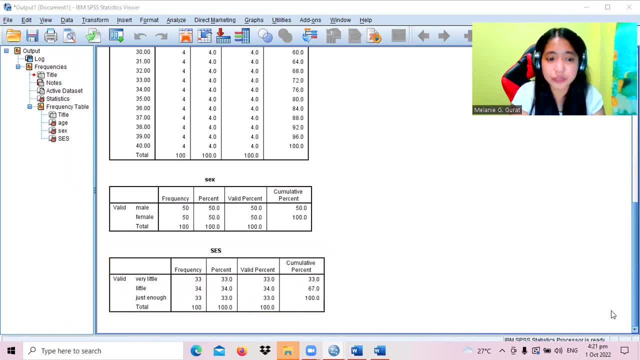 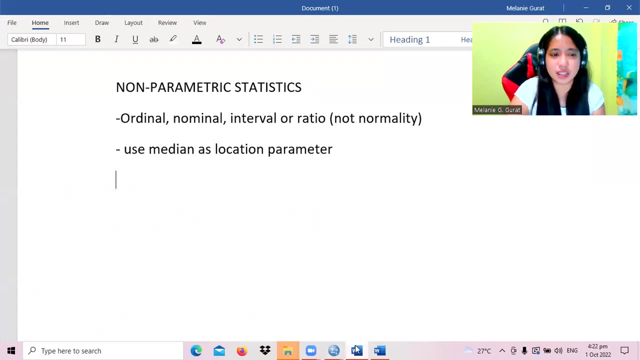 So we have 50 male, 50 female, and then we have very little, little or just. So if we will be using this data, of course we will do the preliminary analysis And our data is at least interval or ratio, because it's numerical. 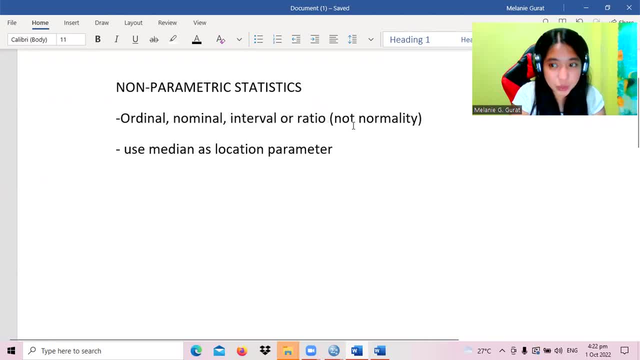 But since it is normally distributed, so let's raise the possible problem: Is there a significant difference in the level of life satisfaction when grouped by- Let us not consider age, because we have two. Okay, So for the meantime we will be answering: is there a significant difference in the level of life satisfaction when grouped according to SIF and when grouped according to socioeconomic status? 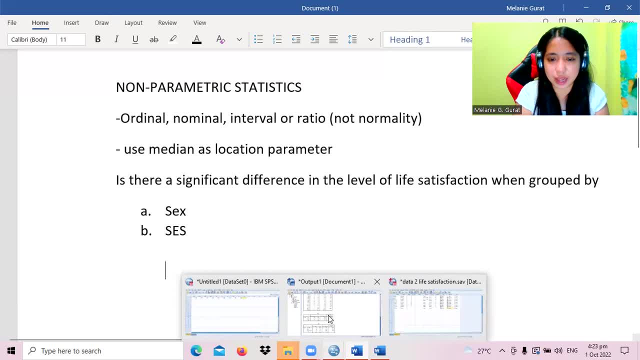 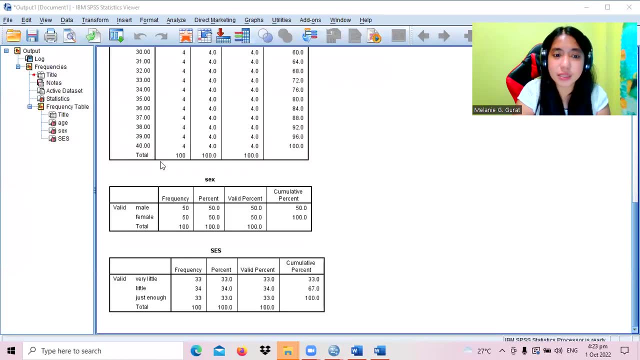 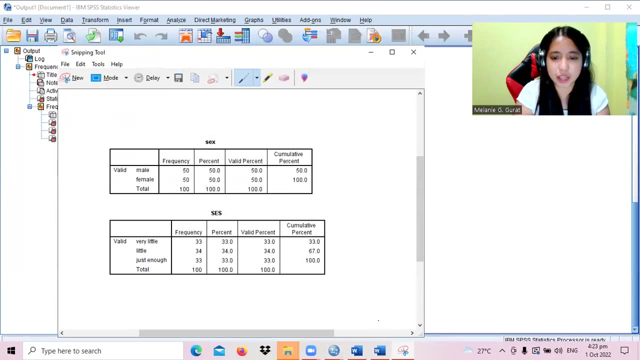 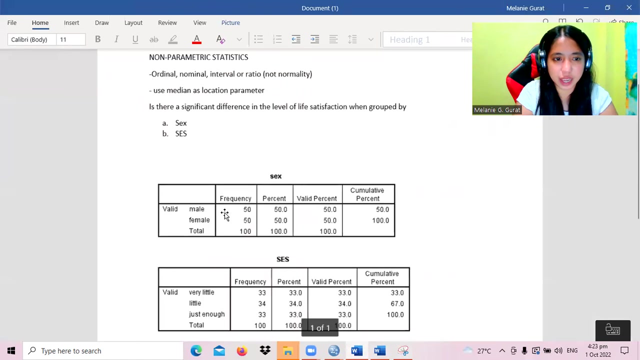 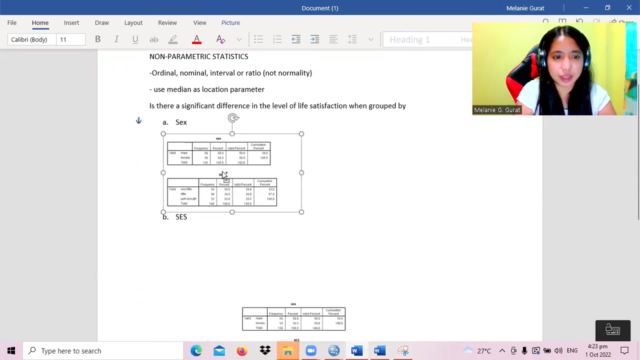 And by looking at the initial data, do you think it is possible, or we can already see that, So we can already conclude that the appropriate measure or the appropriate, rather, test that we can use here is a parametric, And, of course, the answer is yes. 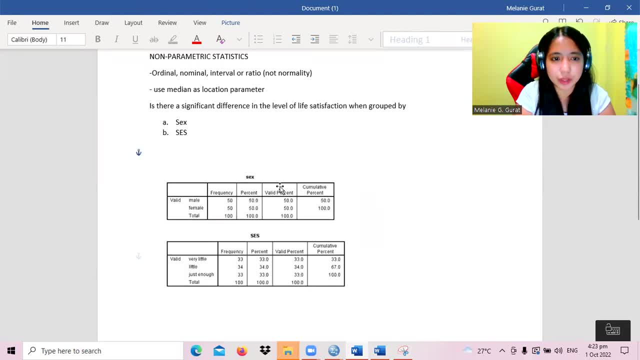 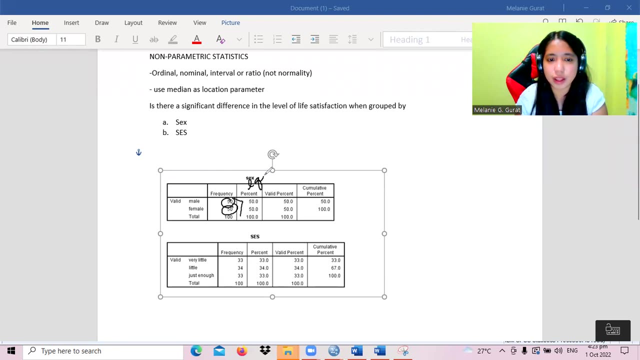 Because by central limit theorem- let me just read this: By central limit theorem, our, Our data is already at least 34 male, at least 34 female, And this for equivalent. So by central limit theorem, our data is normal. 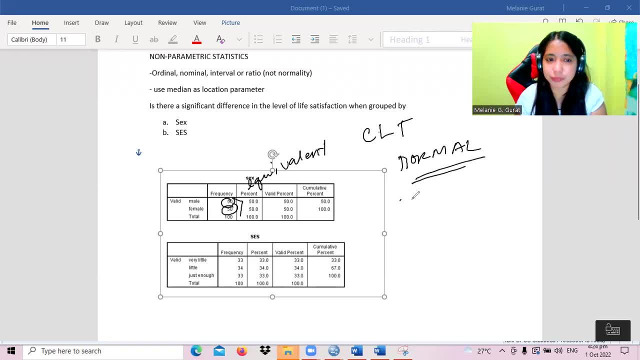 So we will be using parametric test. And then for the second one, so similarly 30-30, it's at least 34 each. Then again by central limit theorem. this is normally distributed And it means that we will be using parametric test. 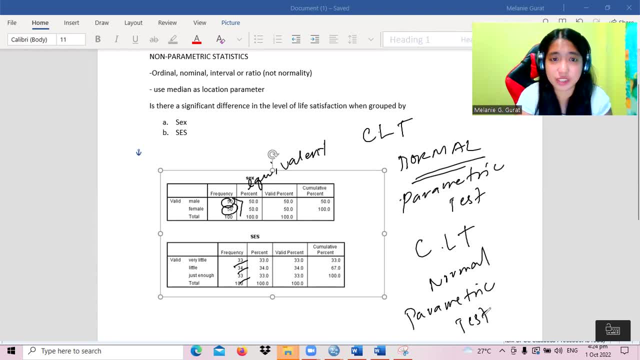 But of course, this is not our objective for this video. Our objective is to use non-parametric test. So which? Which means, how will we use non-parametric test in this problem, Though we know, of course, that the more powerful is the parametric compared with non-parametric? 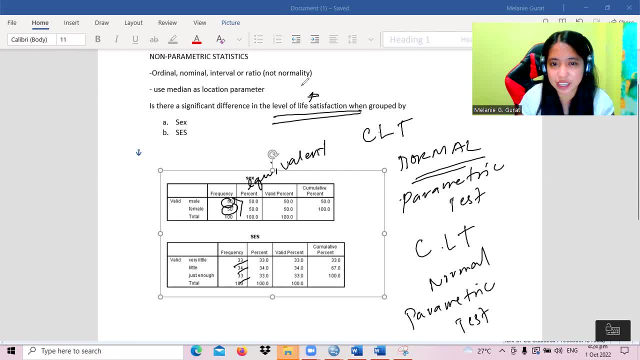 We know that the level of satisfaction generally is an ordinary data. So if I will be using not the scores, not the sum, But the ordinal data, Then even if the data shows that it satisfies the condition of central limit theorem, we cannot use a parametric test if our data is ordinal. 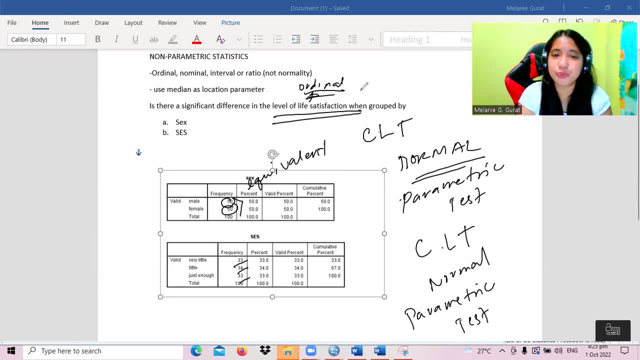 So, assuming that our data is not, we cannot. of course we will not be using, rather we will not be using each sum, But rather we will be using the ordinal. So, going back to our data, Let us just clear our screen. 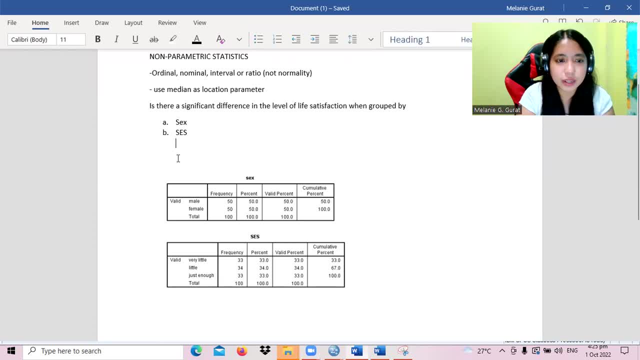 Okay, So going back here, So let's just change the problem. Is there a significant difference in the level of satisfaction in item 1,, for example, when grouped by text? Okay, So let's just change the problem. 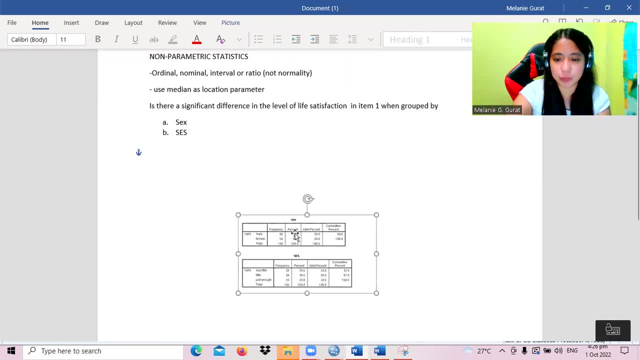 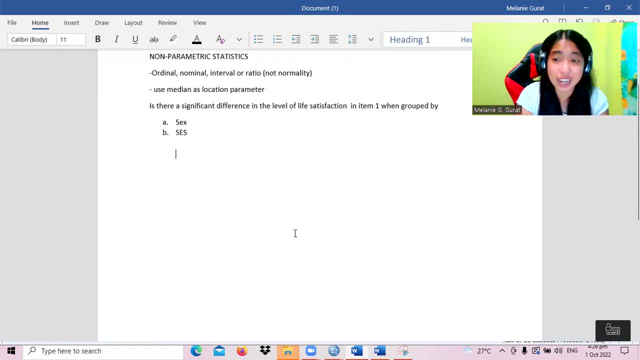 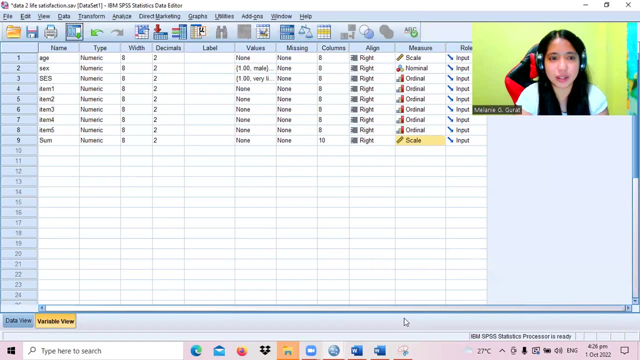 Or, if not, we can also get what is the level of life satisfaction generally not using the sum. And how will we do that? Because, of course, item 1 is ordinal until item 5 is also ordinal. How will we determine if our 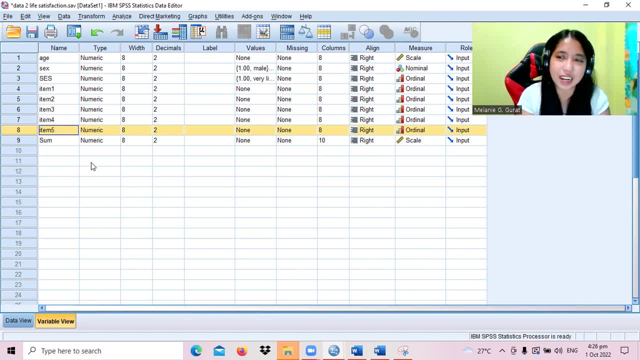 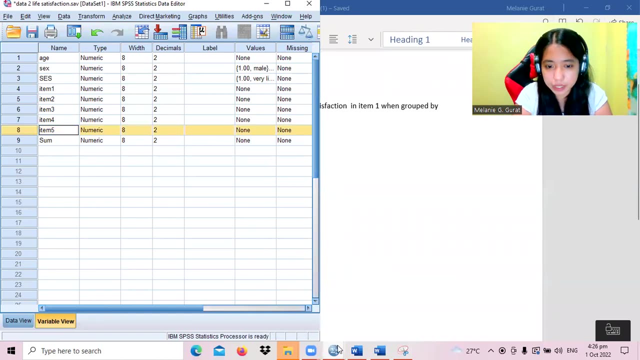 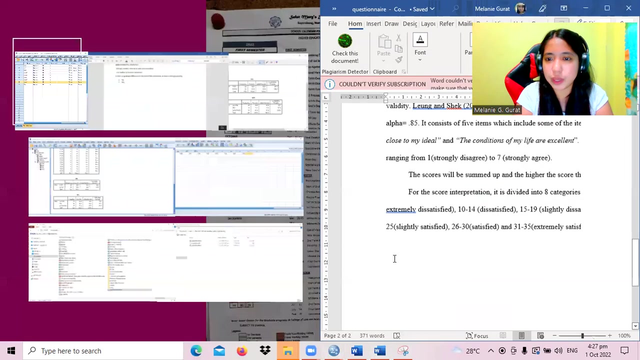 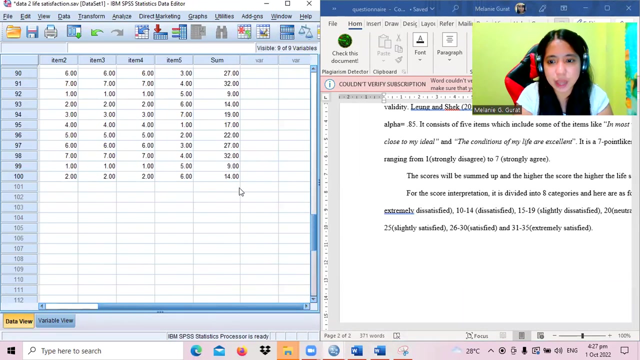 transform. is ordinal data now satisfies or is can be, can be solved rather using a non-parametric. so let us do a transformation, so we will be. let's go back to our data, at our questionnaire record. so we are going to classify the means, or rather this time like, for example, if it is 14. 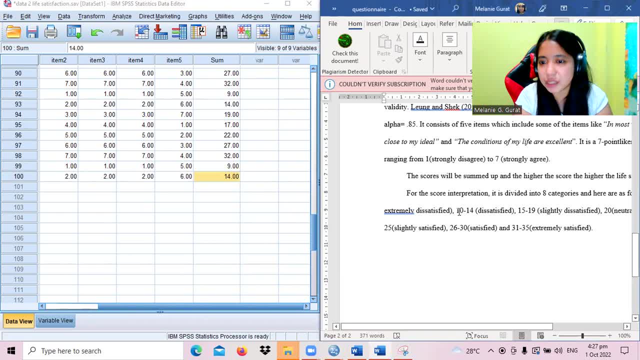 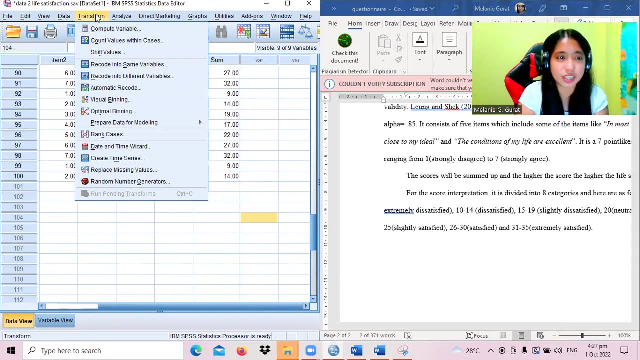 so let's check in our list. so 14 means this satisfied. so we are going to use the organized data. so let's do it to transform. so we are going to use the function of sps a, which is the transformation. we usually use this when we are doing descriptive statistics. 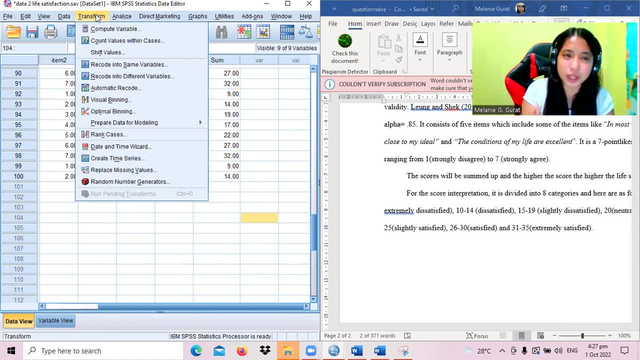 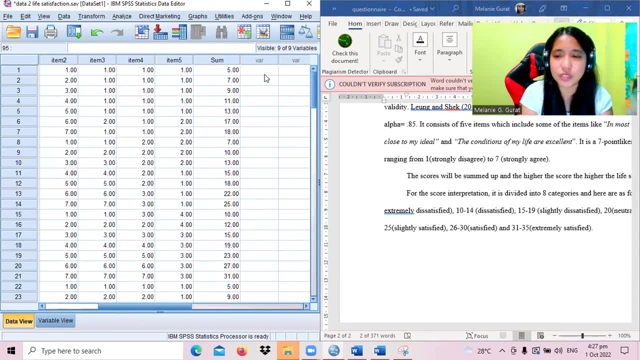 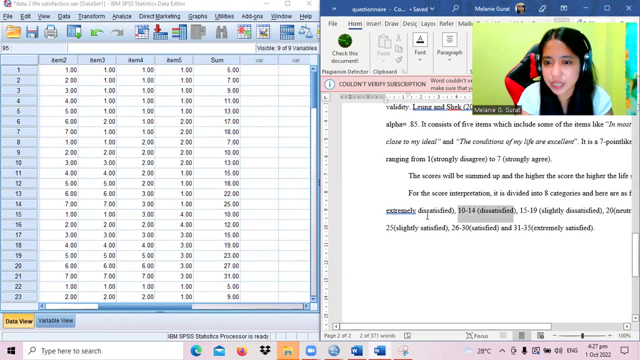 and of course, we can also do it manually, just as i have mentioned. you can classify this into or you can use a coding scheme like, for example here: five to nine. so five is extremely dissatisfied, so i place one here and then this is also dissatisfied. nine is also extremely. 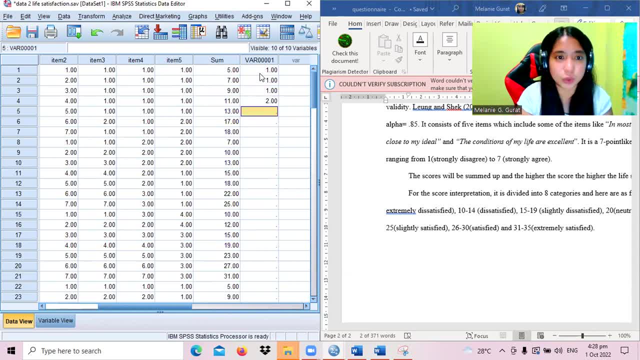 dissatisfied. eleven is dissatisfied, so it's equal to two. you can actually do a sorting, so let's just sort this first. okay, so that is very easy for us to place one for all numbers that is within. okay, okay, so that is very easy for us to place one for all numbers that is within. 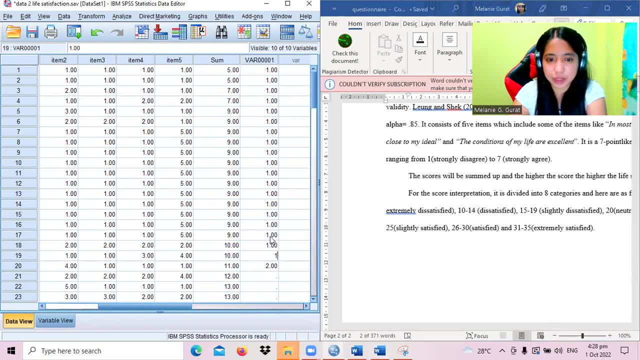 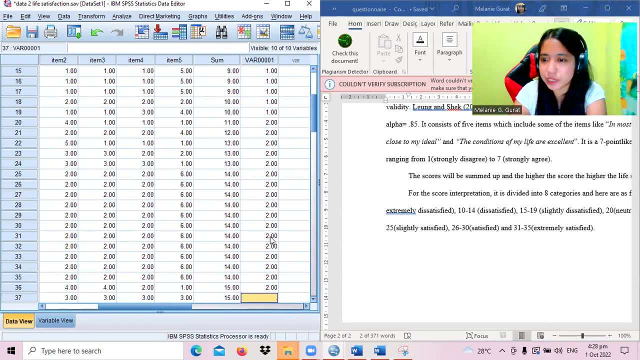 five to nine, and then let's give two for 10 to 14, and when we reach 15, let's just give it a value of three, because of course this means that it's already slightly dissatisfied. until 19, okay. when we reach 20, it's. 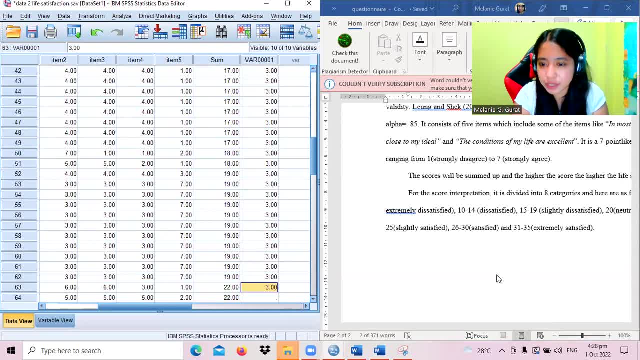 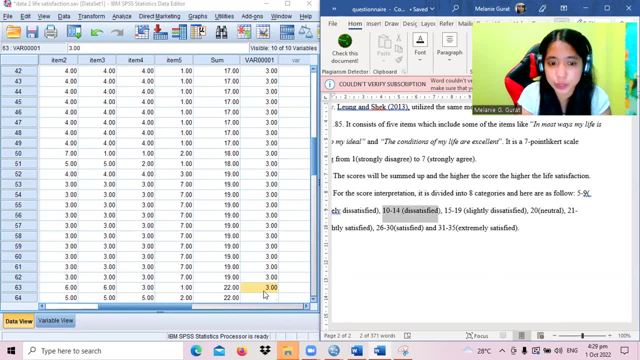 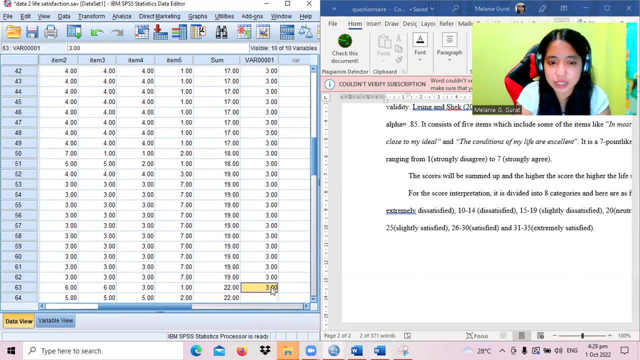 neutral, and let's move here. but if it reached 21, so we do not have neutral, we do not have 20, but if it, if we reach 21 until 25, it is slightly satisfied. so it's four for neutral, five or slightly satisfied, so let's use five until two. 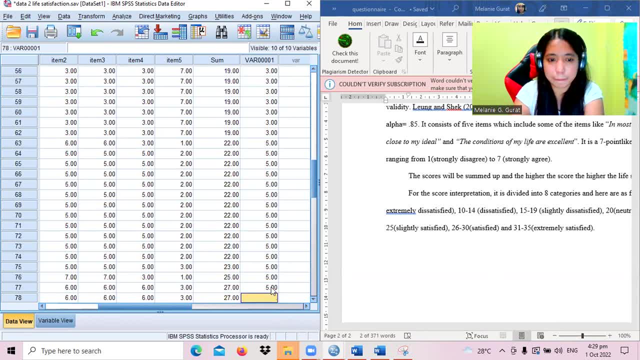 uh until 25.. uh, 27, 26 is starting 26. let's uh 27: 26 is starting 26. let's uh 27: 26 is starting 26. let's place it until 30.. place it until 30.. place it until 30.. when we reach 31 to 35, it means that 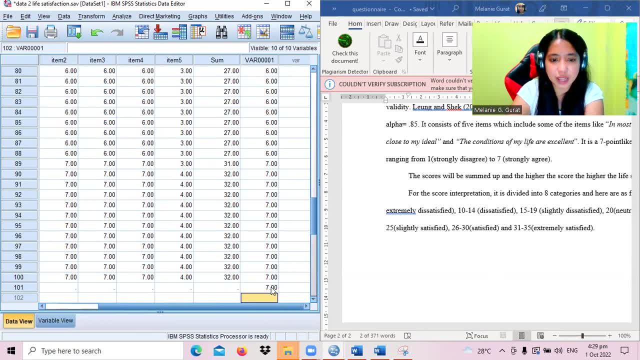 when we reach 31 to 35. it means that when we reach 31 to 35, it means that it is extremely, it is extremely, it is extremely satisfying, satisfying, satisfying. so we are already done placing, so we are already done placing, so we are already done placing our variable. 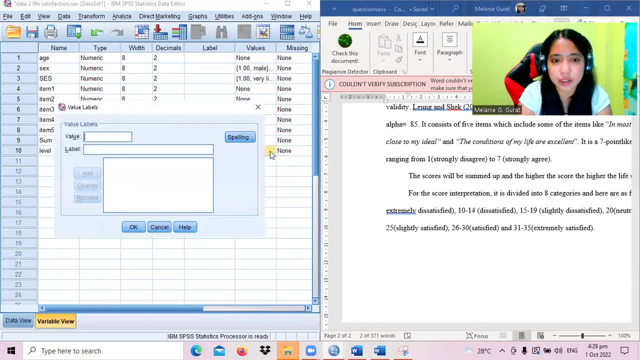 our variable, our variable flip and what is this level flip and what is this level flip and what is this level? so let's place it in the value one means. so let's place it in the value one means. so let's place it in the value one means extremely. 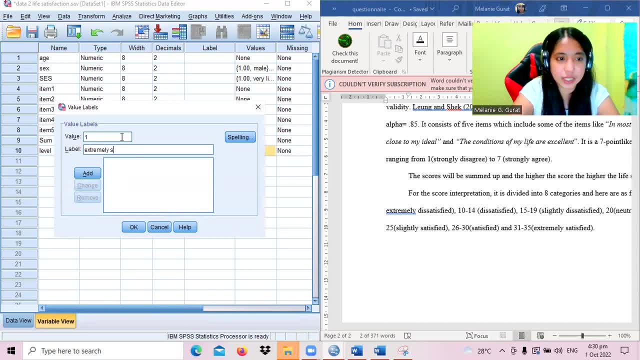 extremely, extremely satisfied, satisfied, satisfied. uh, i mean this: satisfied. who is? who is who is satisfied, satisfied, satisfied? three is slightly, three is slightly, three is slightly satisfied, satisfied, satisfied, four, four, four is four is neutral, but we do not have four neutral, but we do not have four. 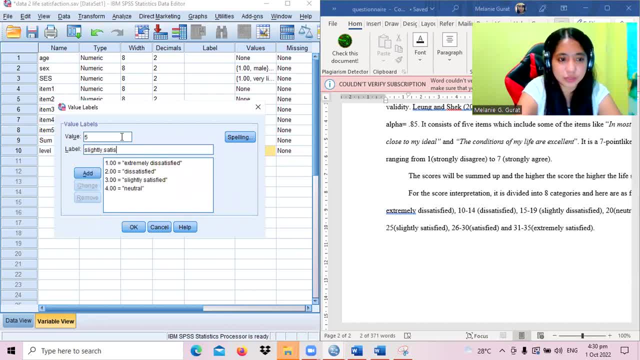 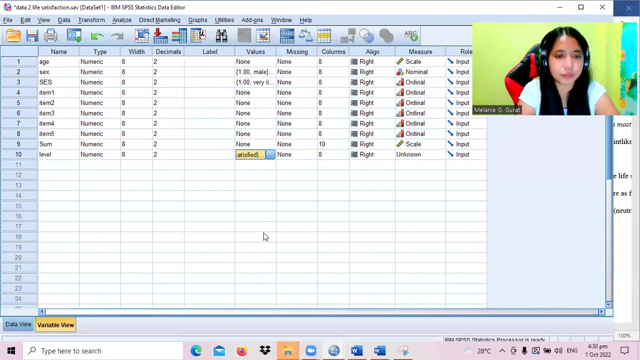 four, four, five is slightly satisfied and six is satisfied and six is satisfied and six is satisfied. seven is extremely satisfied and click okay satisfied and click okay satisfied and click okay. so this is now our data. so this is now our data. so this is now our data. so, going back to our problem, 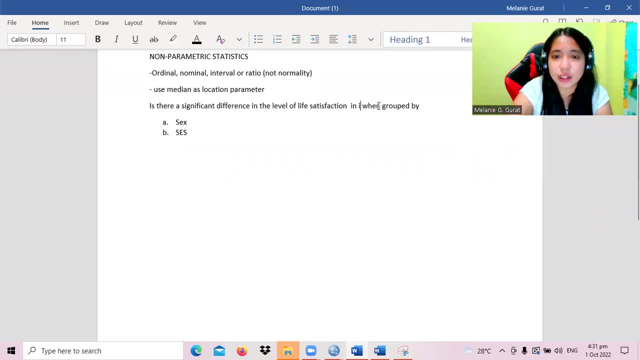 so going back to our problem. so, going back to our problem, is there a significant difference in? is there a significant difference in? is there a significant difference in the level of the level of the level of satisfaction when group one satisfaction when group one, satisfaction when group one? if just in case, 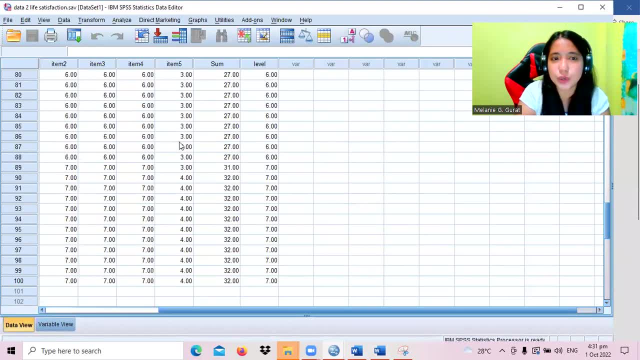 if just in case, if just in case we do not have, we do not have, we do not have. if just in case we do not really have, if just in case we do not really have, if just in case we do not really have the data on some and what is accessible. 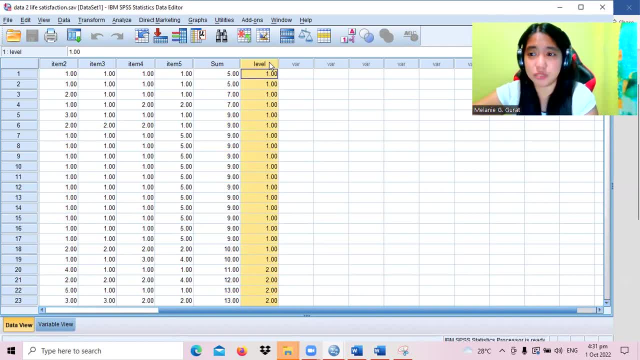 the data on some and what is accessible. the data on some and what is accessible to us. is the data only for level of to us? is the data only for level of to us? is the data only for level of satisfaction, satisfaction, satisfaction, the ordinal data, then it. 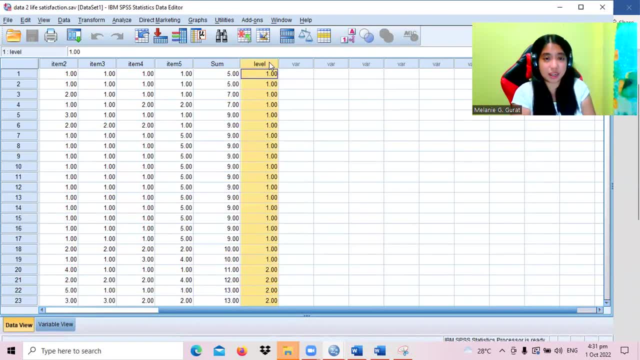 the ordinal data, then it the ordinal data, then it means that we cannot use a means that we cannot use a means, that we cannot use a parametric test. we cannot parametric test, we cannot parametric test. we cannot consider parametric tests instead. we consider parametric tests. instead we. 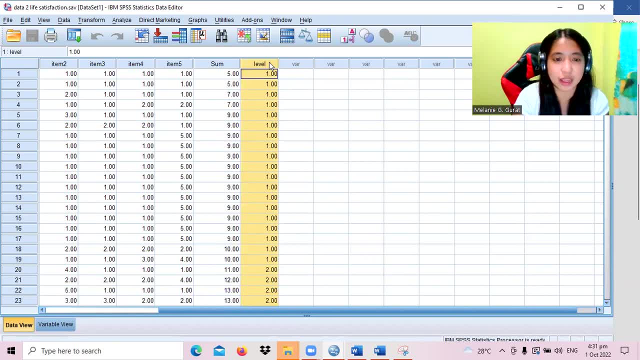 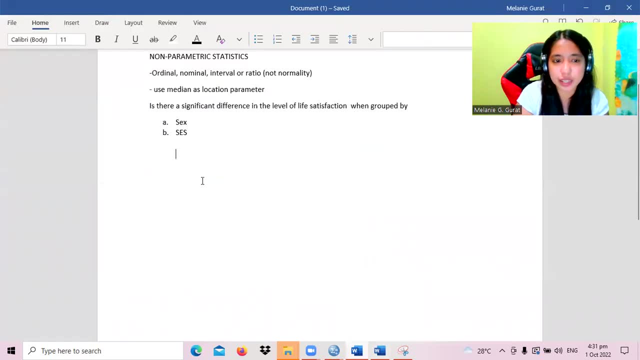 consider parametric tests instead. we can use now the non-parametric, can use now the non-parametric, can use now the non-parametric. so how to so, how to so, how to generate the. generate the. generate the table that will answer this table. that will answer this. 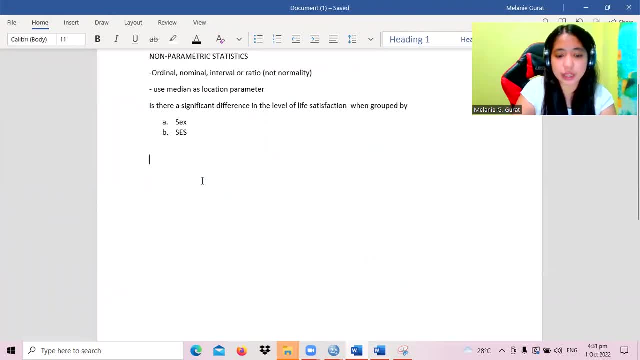 table that will answer this. so, so, so, the, the test that is used to answer the, the test that is used to answer the, the test that is used to answer this, this, this. so this is a comparison, so this is a comparison. so this is a comparison of. 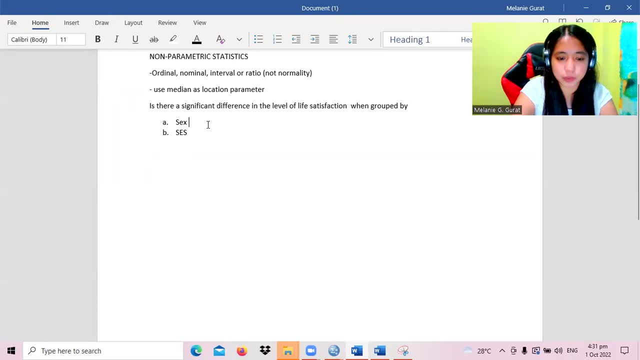 of of for letter a. it's a comparison of for letter a. it's a comparison of for letter a. it's a comparison of ordinal data grouped. ordinal data grouped. ordinal data grouped by two categories. so we will be using man, so we will be using man, so we will be using man with me. 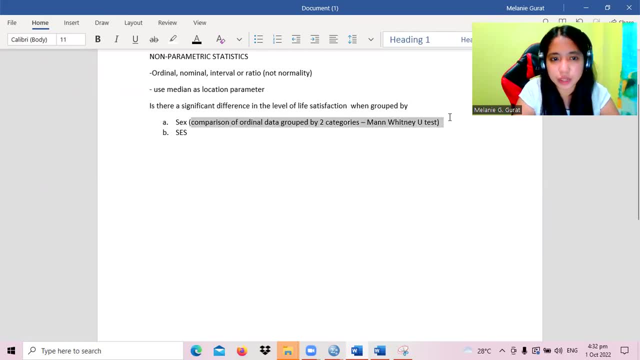 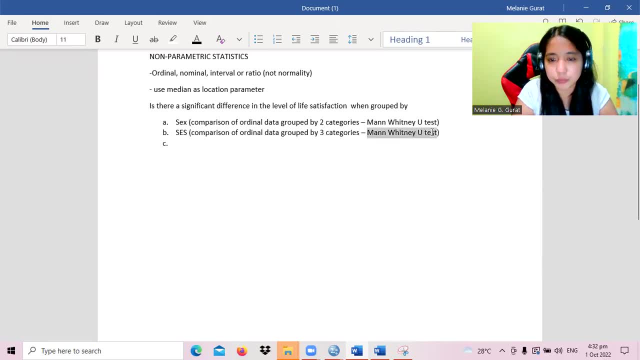 a comparison of ordinal data when grouped. a comparison of ordinal data when grouped by three categories. we will be using by three categories. we will be using by three categories. we will be using crystal, crystal, crystal, white and, in case, white and in case white and in case that the result. in case that the result. 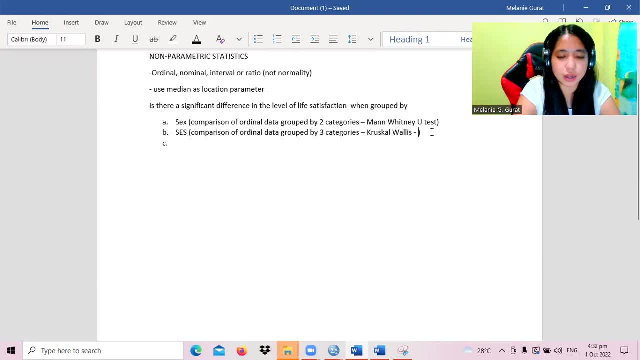 that the result, in case that the result, that the result, in case that the result is significant, we will be- is significant, we will be- is significant, we will be using pairwise, using pairwise, using pairwise, comparison, comparison, comparison if result is, if result is, if result is significant. so, just like anova, we use 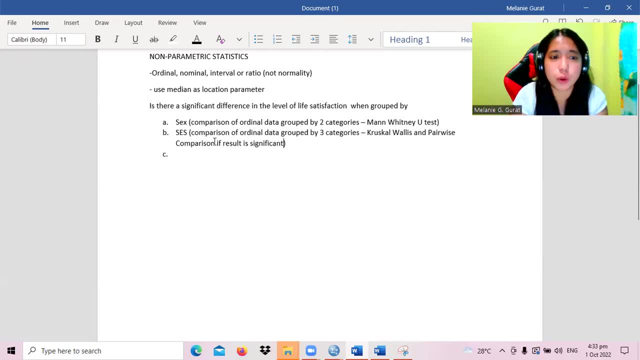 significant. so just like anova, we use significant. so just like anova, we use bonferroni or chipe, or bonferroni or chipe, or bonferroni or chipe, or postbox comparison. so we are now ready. postbox comparison. so we are now ready. 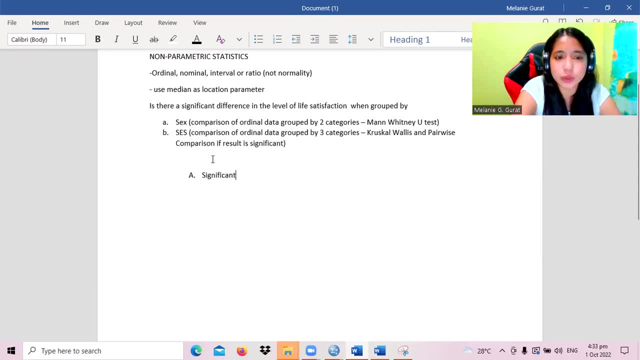 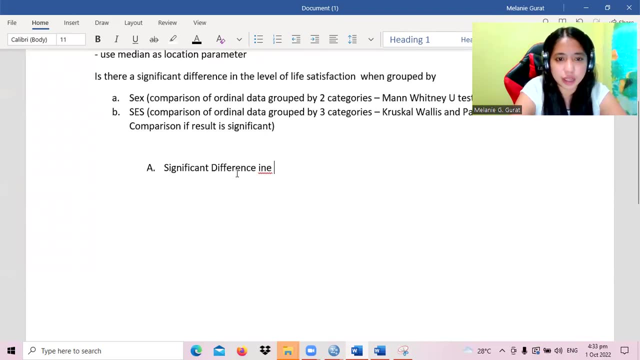 postbox comparison. so we are now ready to answer, to answer. to answer letter a. so the table that we'll be letter a, so the table that we'll be letter a, so the table that we'll be presenting, and presenting, and presenting, and the significant difference, the significant difference. 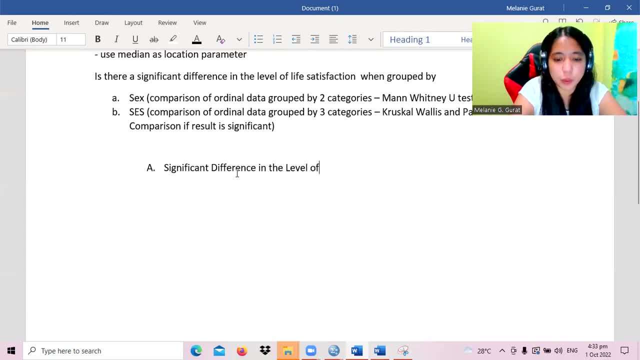 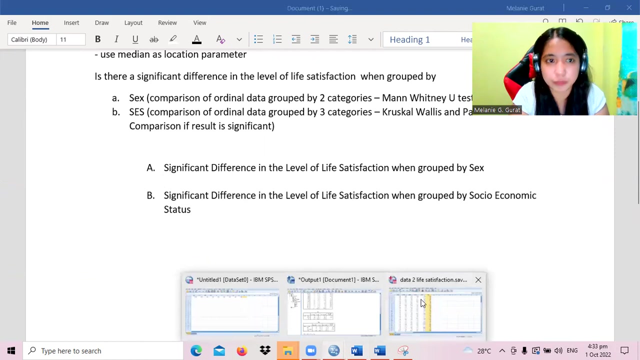 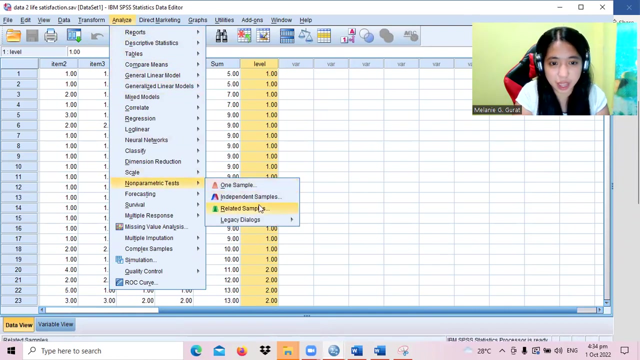 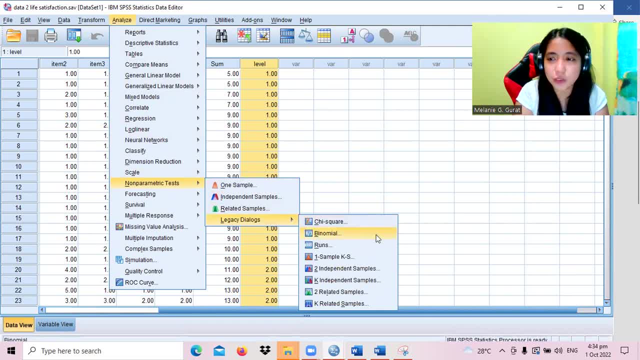 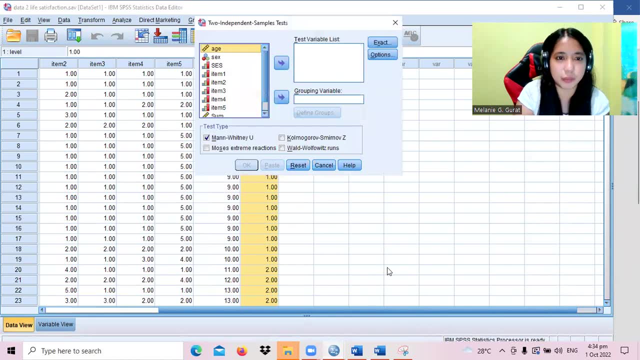 legacy dialogue and, of course, male and females are independent, so we will be going to independent sample. Let's transfer our level as test variable, so this must be an ordinal. So we failed to change. and when grouped according to set. So we will be defining this: 1,, 2, and 3.. So look at this so we actually have other. 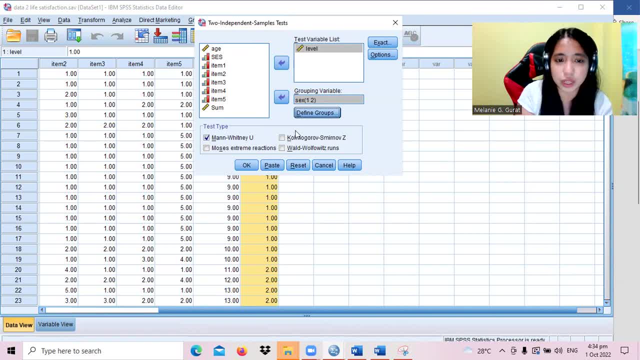 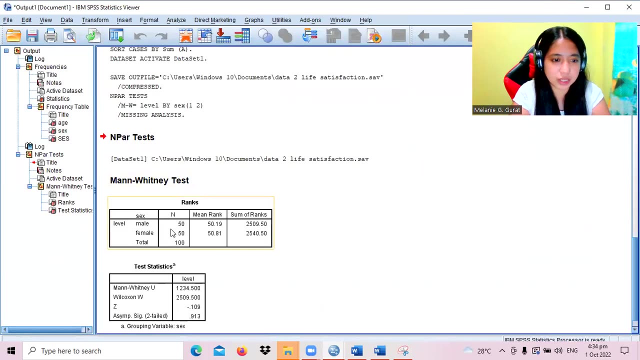 more tests aside from Mann-Whitney. So we have Mortis, Extreme, Kolmogorov-Smirnov, Waldkowitz and Handel, So of course we will be using Mann-Whitney, which we will then click OK. So this is now the result. So when 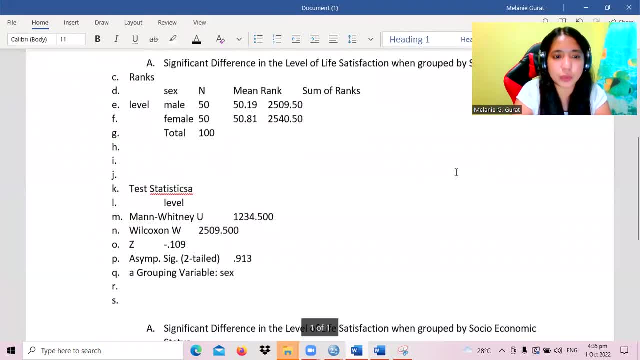 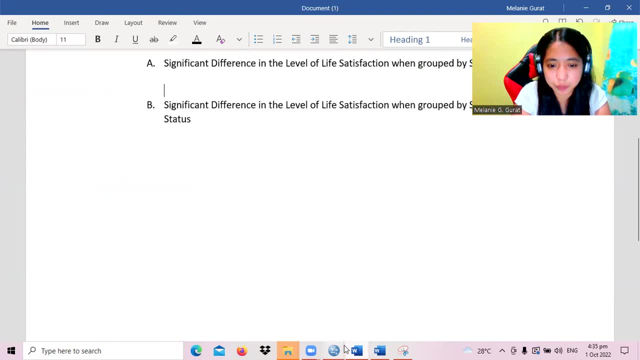 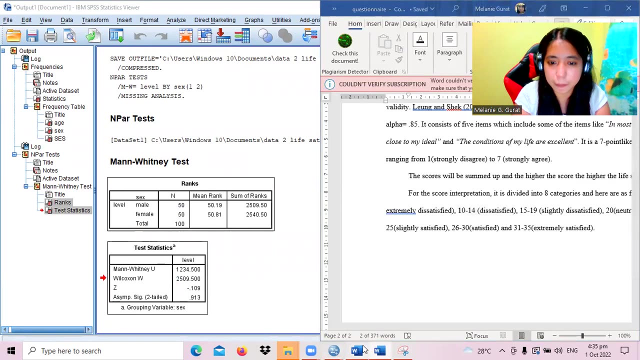 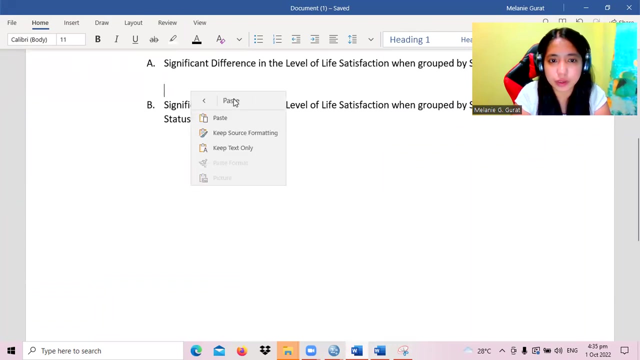 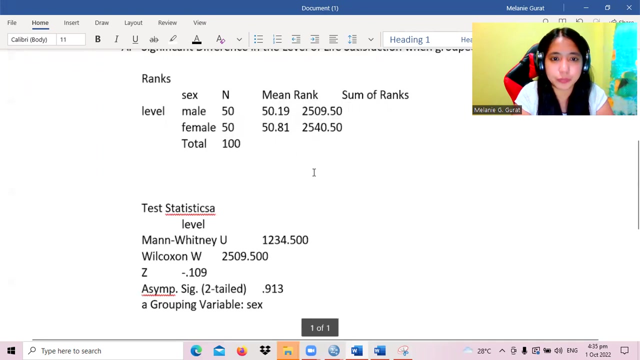 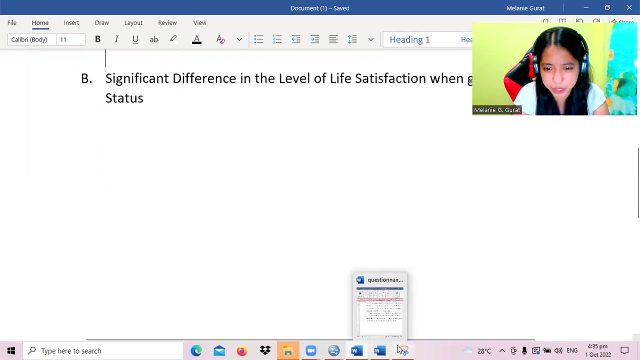 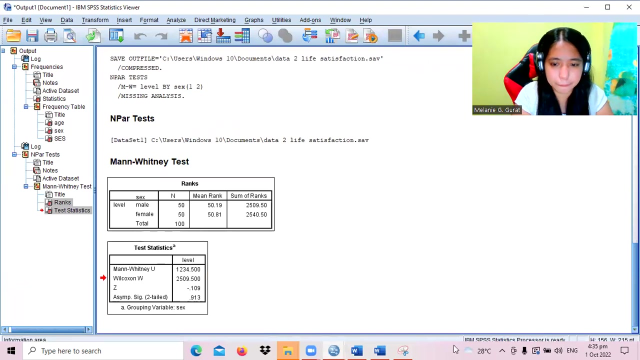 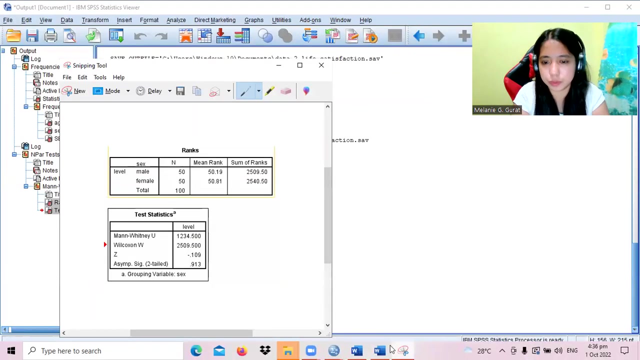 interpreting this table. it is just similar with how we let's just get with the first test, So let's go ahead and see if we can get it to the table, Or maybe let's just get it to the first test And if we will be presenting this. 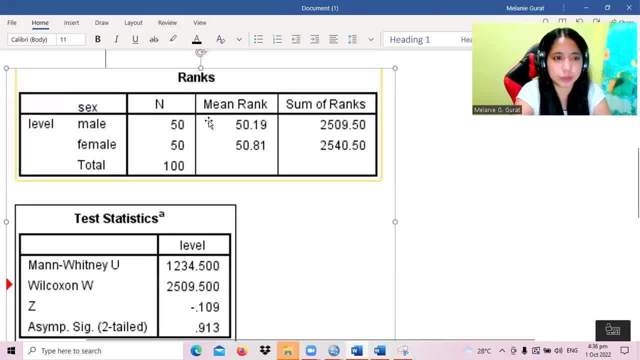 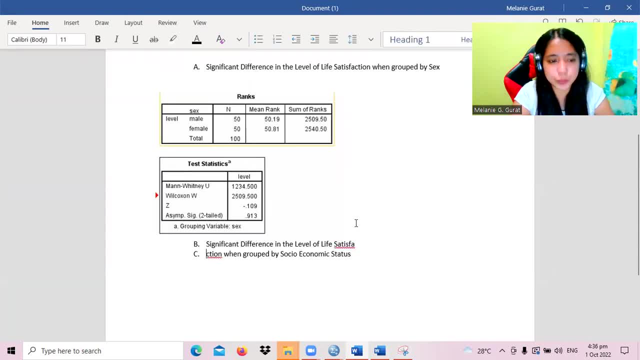 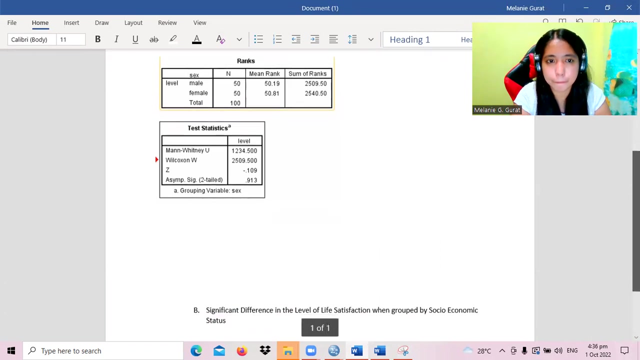 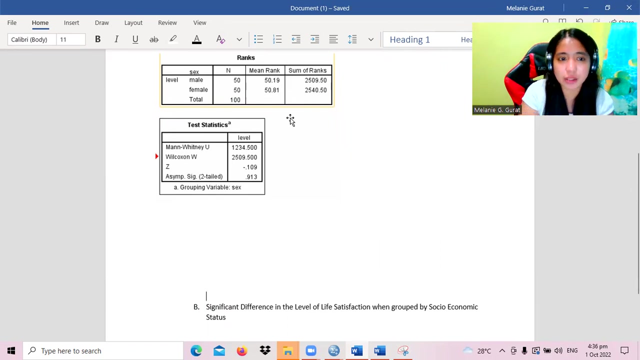 And if we will be presenting this. And if we will be presenting this, We just need to present and mean rank, sum of ranks, And it's okay not to present the result of both, So we can just proceed to Mann-Whitney. So let me just show it here. 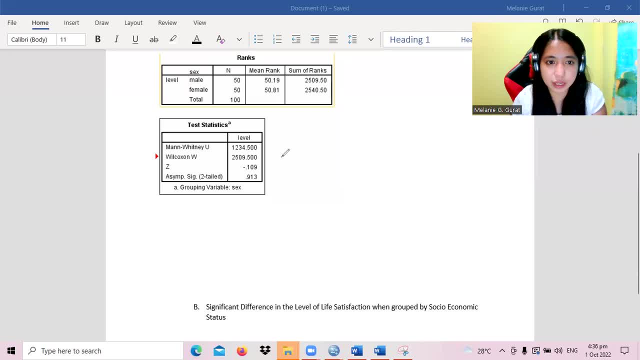 So we can just proceed to Mann-Whitney. So let me just show it here. So we can just proceed to Mann-Whitney. So let me just show it here. So, if we will be presenting this, So what will be the table? 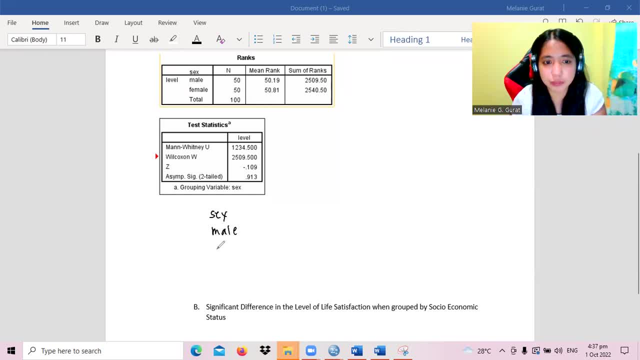 So set male, female and then N. It's your option if you also would like to present the median instead of the mean rank, But anyway, But anyway. But anyway, If we use the mean rank, it also means the same thing. 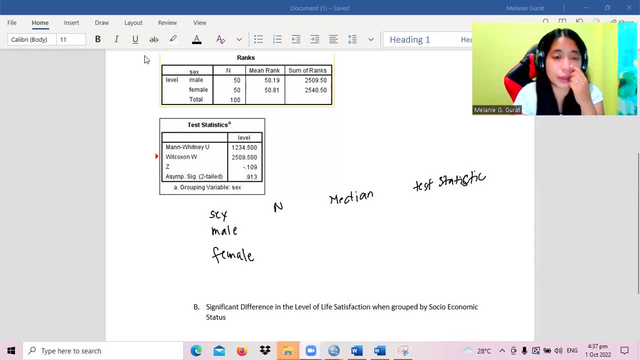 So the higher mean rank means the higher mean And lower mean rank, the lower the value of satisfaction. So the symbol for test is U because this is Mann-Whitney U test. So the symbol for test is U because this is Mann-Whitney U test. 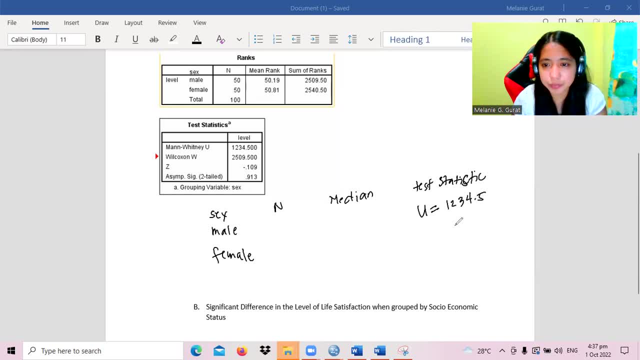 U is 1234.5.. And P is equal to 0.913.. we can just copy the value here or this is all. you can also use the meaning. so using this, of course, is it can be said that the satisfaction of female is. 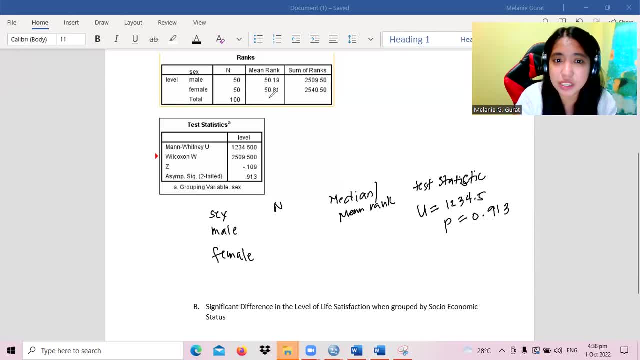 higher than the satisfaction of male because it has higher minimum. however, the result of you test- and with me you test- reveals that the result is not significant. so the level of satisfaction of male and female are the same, regardless or other. the level of satisfaction of the respondents are the. 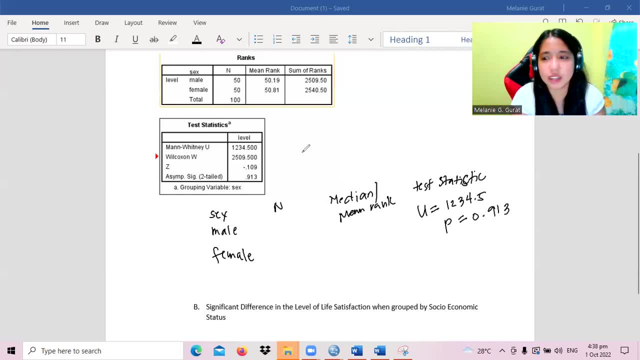 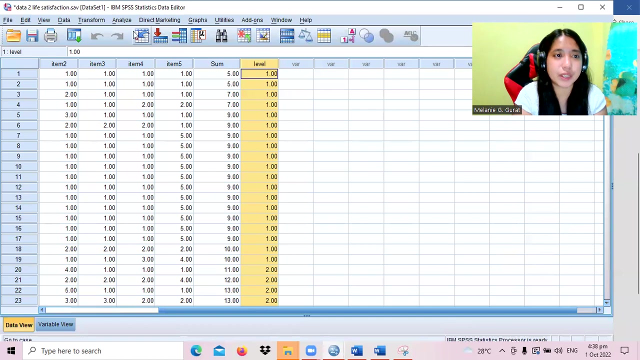 same, regardless of your test. so that is what it means. now, moving to the next example. so since socioeconomic statuses group accordingly into three, then it means also that you cannot use man with me, you test. therefore, what we will be using is crystal value analyze, then parametric test. 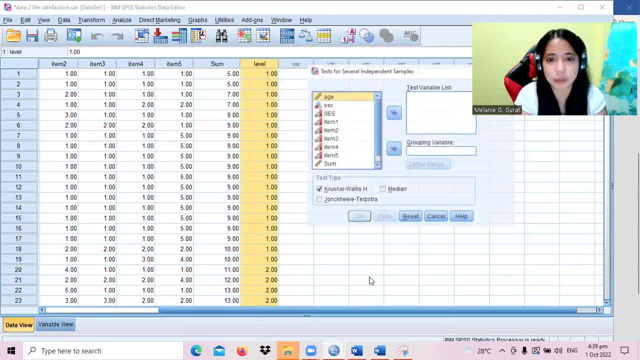 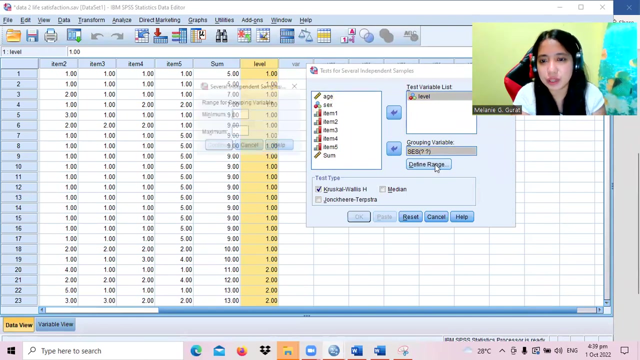 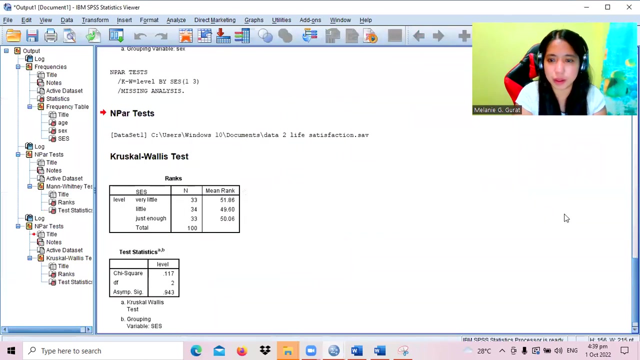 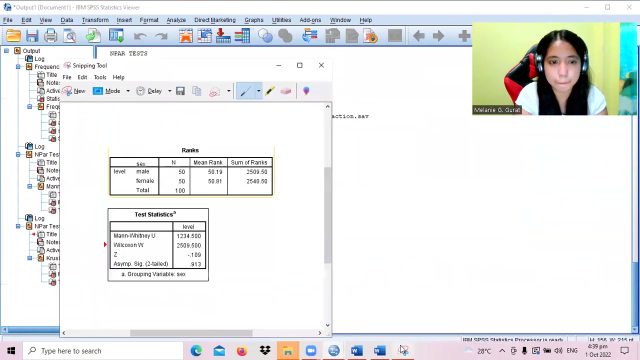 you just see dialogue, a independent sample. so we will be placing the level as mentioned because we are using the original data. for that we are using non-parametric and socioeconomic status, so the number here minimum is one. maximum in the result is also not you, you, you. 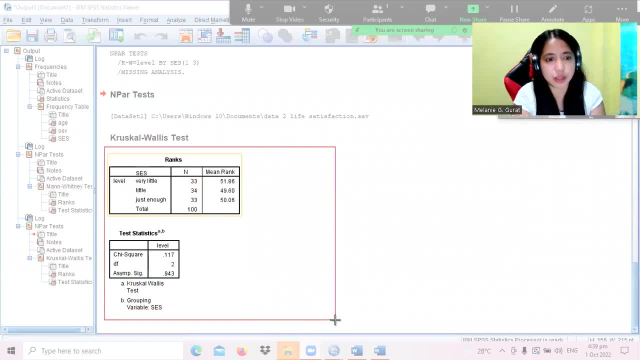 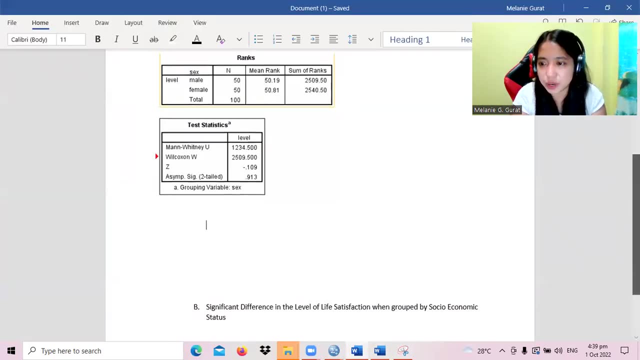 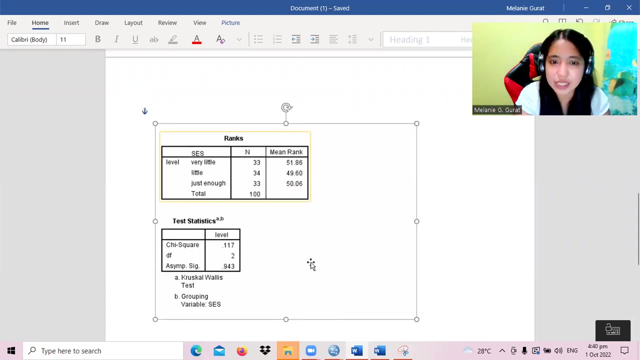 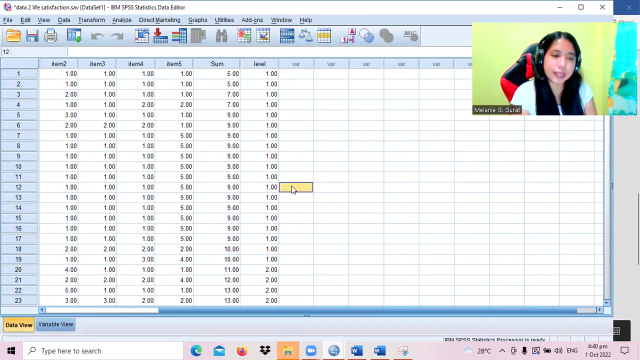 you the result? so what if? what if? let's say that the result is significant? so where can we find? where can we find the pairwise comparison? so in case that, or maybe we can just edit our table and try to work also on samples. that shows a a. 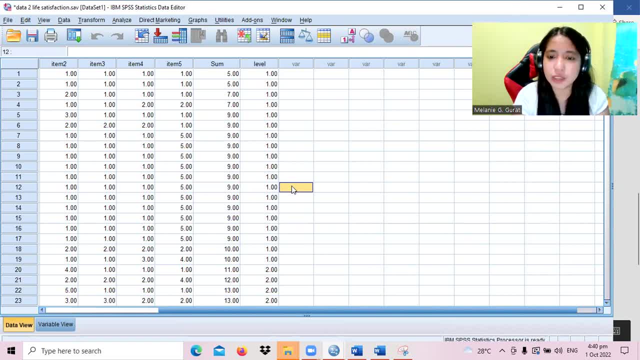 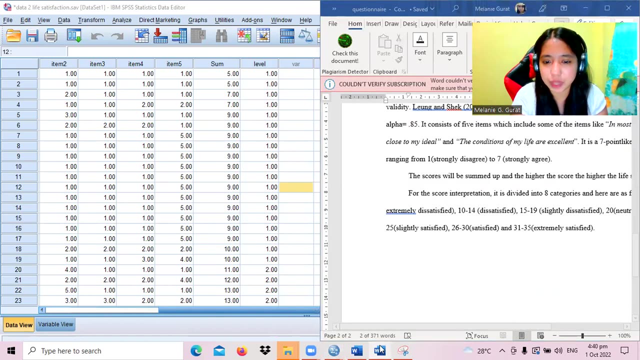 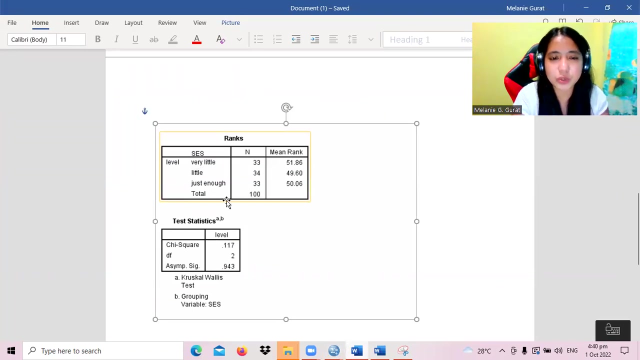 significant result. so maybe in a separate video we will be presenting another example of a crystal wireless generating crystal wall. is that will show a significant result? okay, let's just go back here. so it also means that the highest are those who belong to very little socioeconomic status, followed by 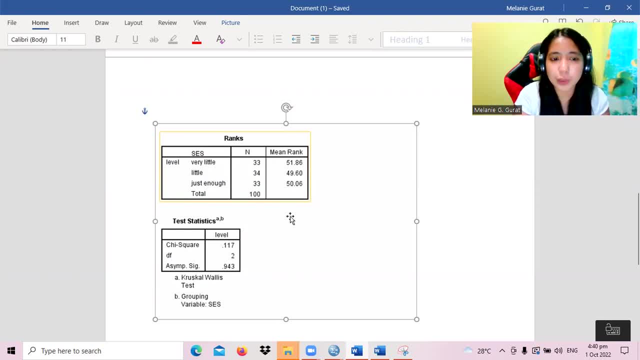 by just enough, and the lowest is that little. however, again, the result of crystal wallis test, the symbol for crystal wallis test, is just the same with the chi square. so it's chi square one. one, seven degree of freedom. two. asymptotic significance is point nine forty. so how is 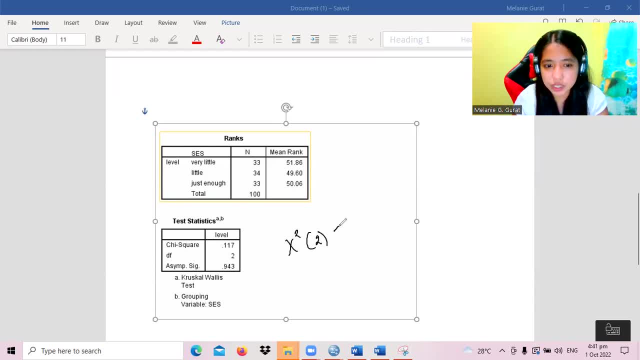 this written. so chi square two is equal to one one seven t is equal to point nine forty three. this is not significant, so the level of satisfaction of the respondent again or the same, regardless of their socioeconomic status. so this ends the video. thank you for watching you.